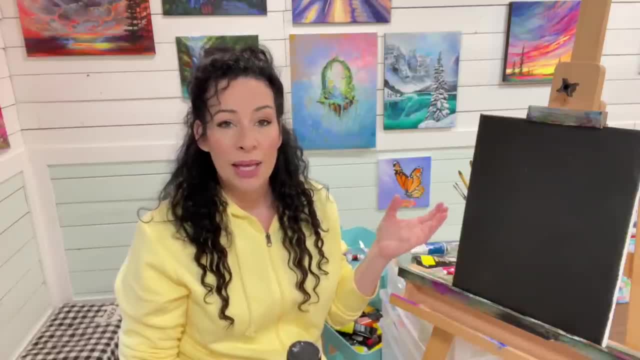 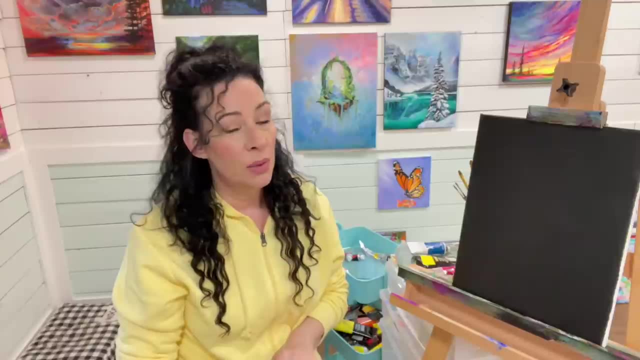 canvas and the paint. It makes it easier to apply the paint. it makes it a little bit smoother. but the main thing for me and the biggest impact I get from the gesso and why it's so important, is: I love color. If you really want your colors to last and not fade, then gesso will do that. 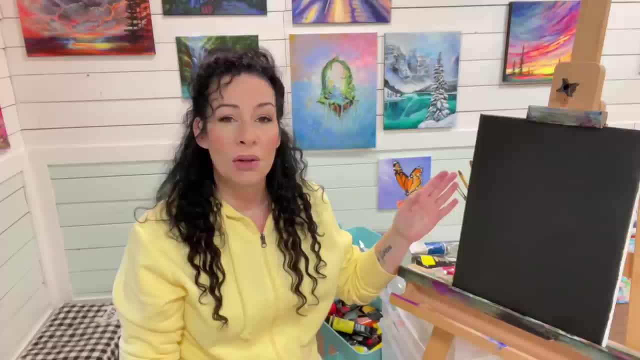 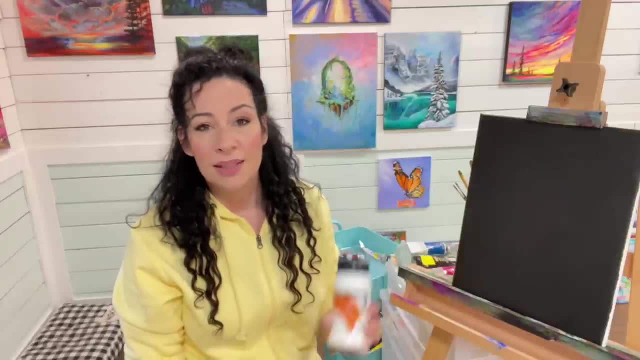 it'll protect that barrier so your paint won't soak into the canvas and dull over time. So if you're having, if you're noticing that with your paintings, try using some gesso and see the difference that'll make. Okay, so number two, that was number. 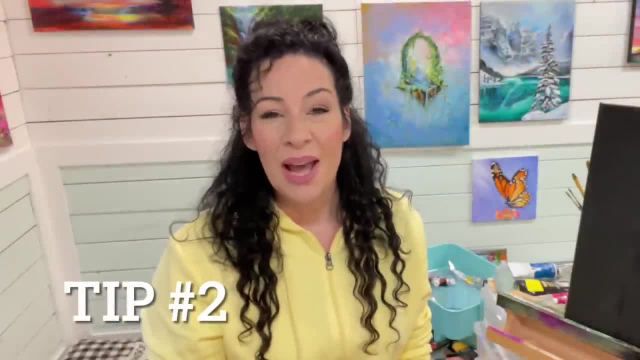 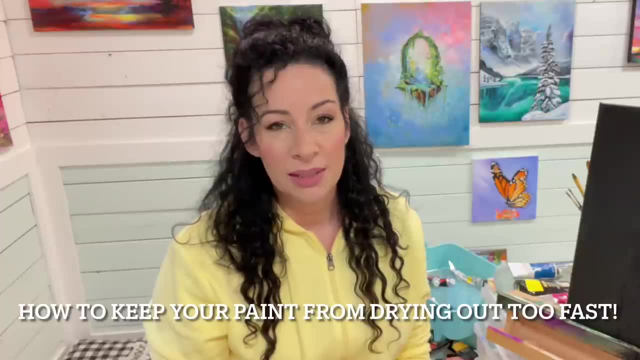 one. now we're going to go into number two. So tip number two: how to keep your acrylics from drying out so fast. I think I get this question more than any other question, and I've got a few different tips for you guys today. So number one: a fine mist spray bottle. You can mist your give a light spray. 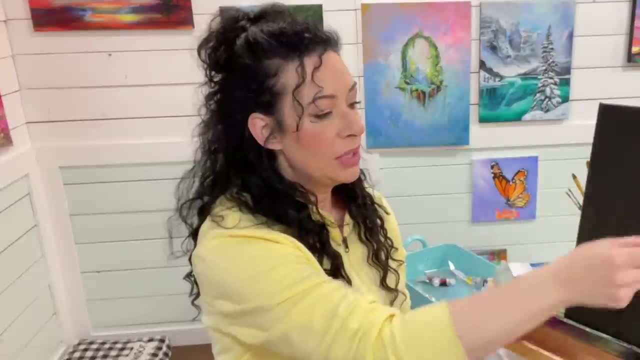 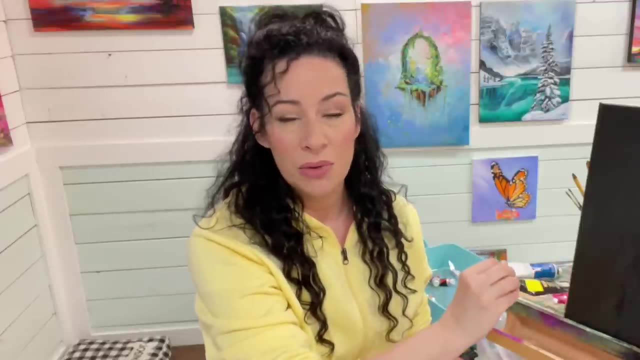 to your canvas and then just kind of spread your whole canvas just with a very, very thin amount. If you're painting off your canvas, that's way too much, your paint is going to be too thin and that won't work unless you're wanting to use watercolors. but you're here for acrylics, so not. 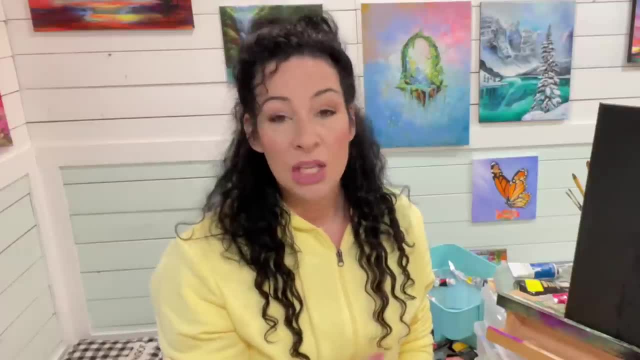 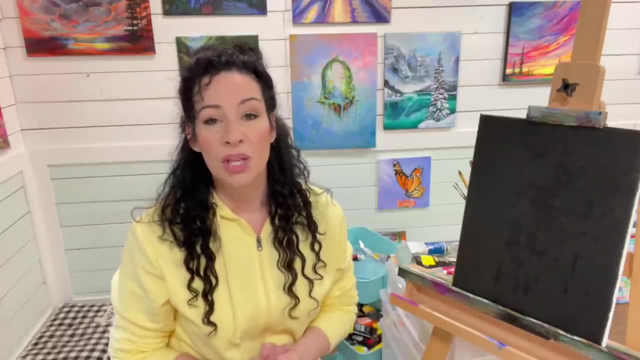 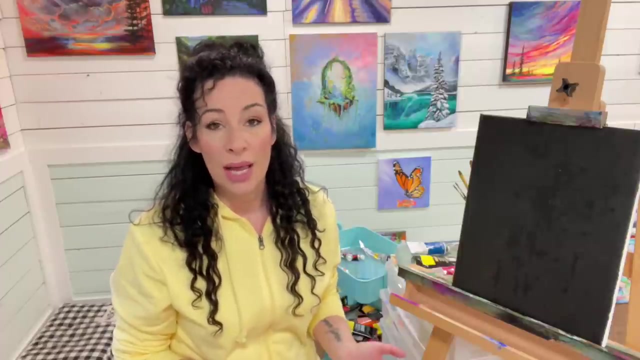 watercolor, So you just want to do a light, thin mist. You want to do that to your palette as well, The other thing that you can try- and, first and foremost, I keep my studio on the cool side and I live on the coast, so the humidity is high here, so it's not dry. That really is a big key in keeping. 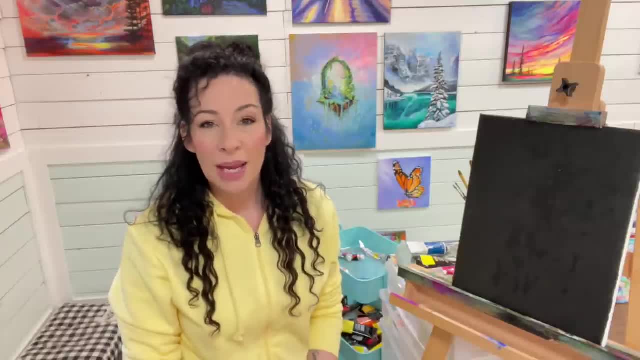 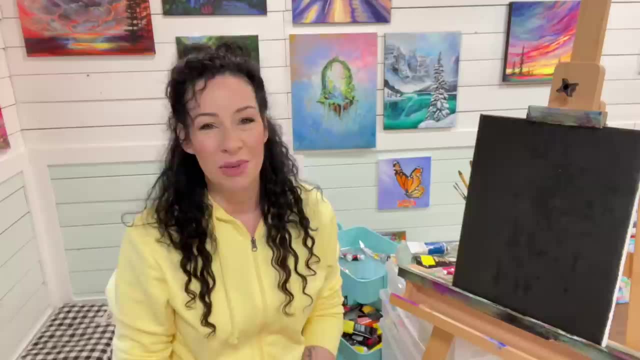 the temperature down in your room. I'm also a fast painter and that's just. I can't help it. I've always been like that. I think it's because I'm so passionate and I'm in that creative flow and I'm really excited while I'm painting. So if you're a slower painter, then what you might want 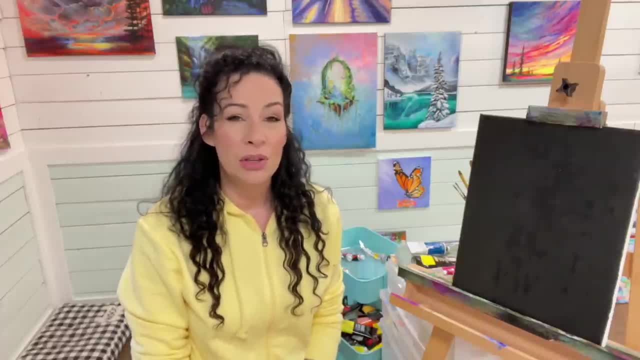 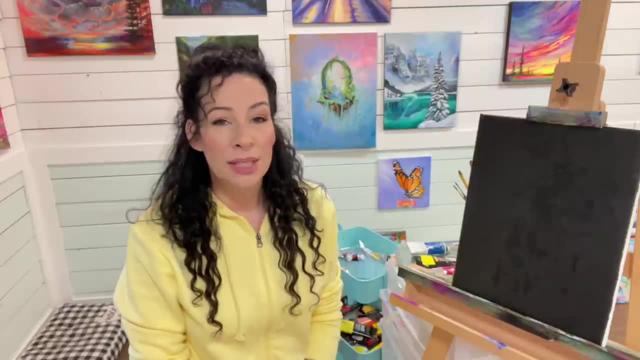 to try. if the water, the spray bottle, is not helping, if the temperature in your studio is not helping either, you may want to try a slow drying medium to add to your acrylics. So that will make your acrylics act more like oils, so it can be helpful for you. 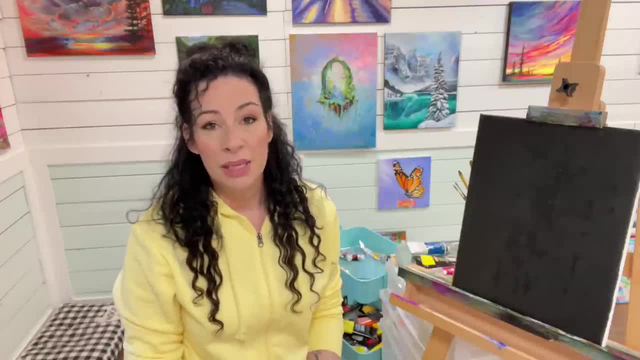 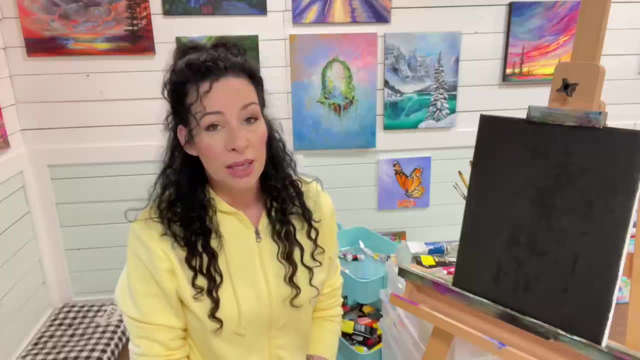 It can be a little bit frustrating and I choose not to use it because I like to be in control of adding my layers, highlights and whatever I want. But when you add the slow drying medium and your acrylic can take hours and hours to dry, it can be very frustrating for the type of painting that 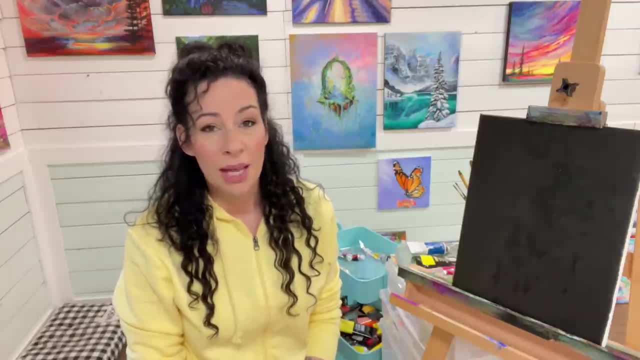 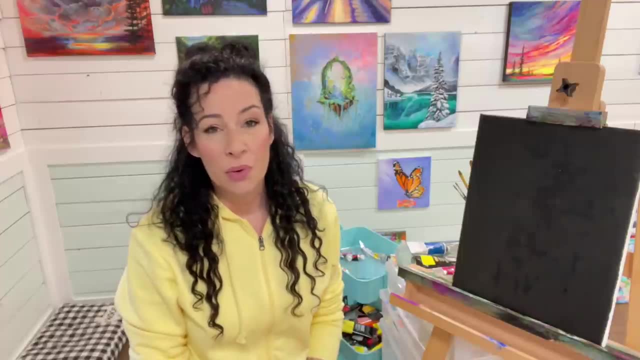 you want to be doing. I like to start a painting and complete it in one day. When I have that vision and that creative mode that I'm in, I don't want to have to stop and wait hours for the layers to dry because by that time my 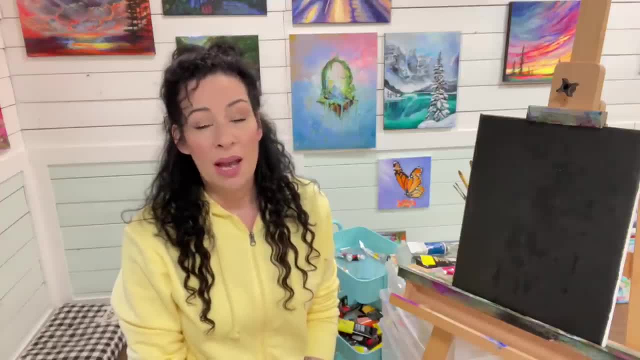 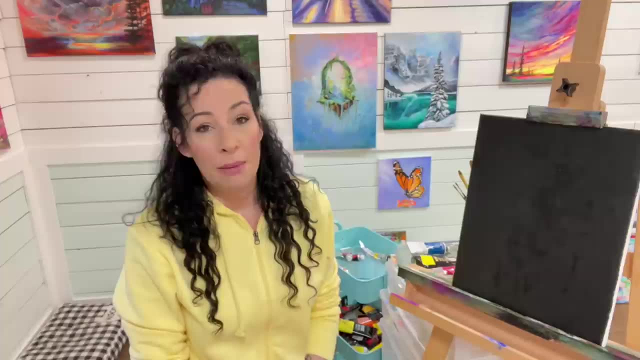 Mood may have changed, my creative flow may have changed and I may have lost that vision and that painting that I was going for or feeling at the time and that can be very hard to get back. So I really like to be in control of my drying time. 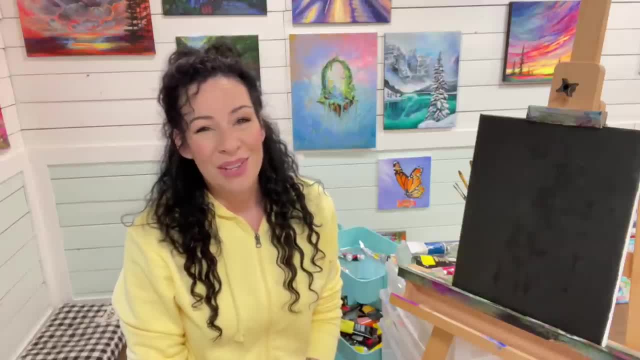 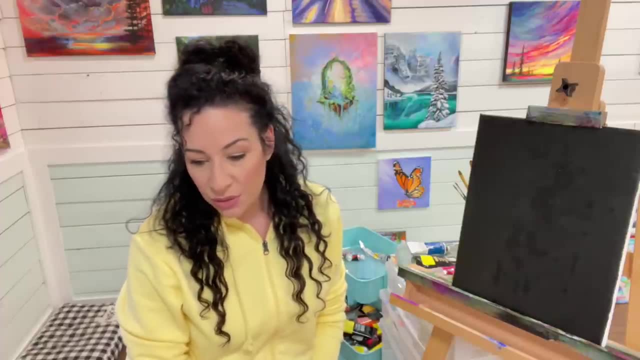 over my acrylics, but it's just something to keep in mind if you guys are using a slow dry medium. But there's so many artists out there that enjoy using it, and another thing you want to do to keep your paint from drying out is when you're finished your painting and when you're never clean up yet if you're finally getting your painting. 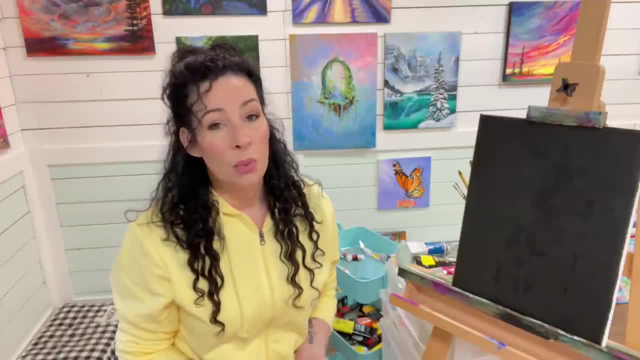 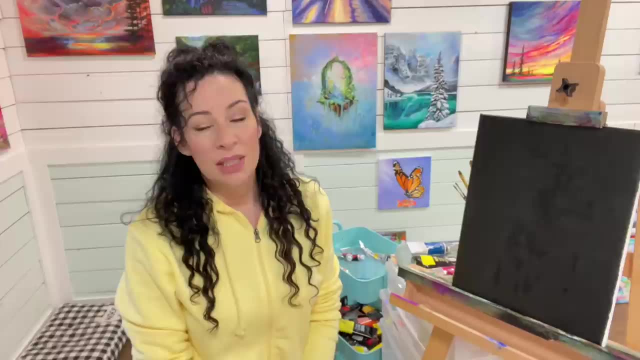 may have a lot of paint left over on your palette. you don't want to waste that, you don't want to leave it sitting out. you can just simply cover it with tin foil, saran wrap, a lid. quite an established artist back of the day gave me this very good tip. he had a little fridge, a little cooler, that he kept all. 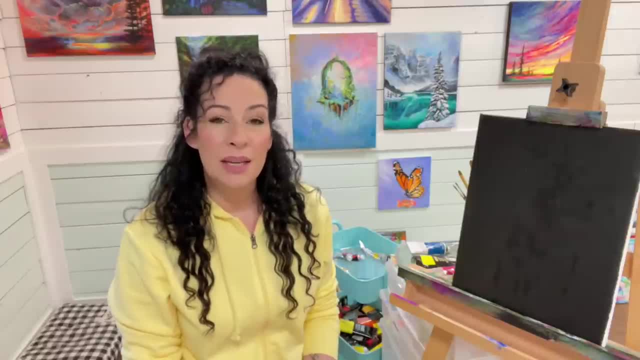 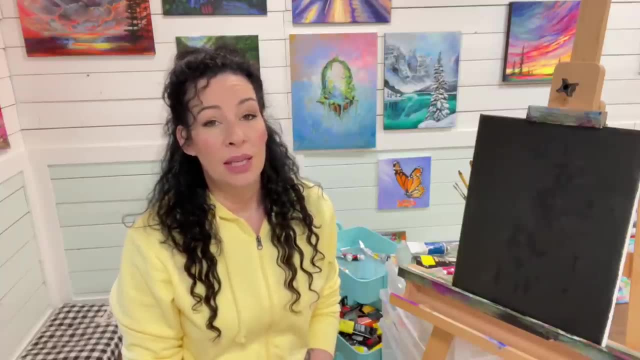 of his paints and from drying out. so you can just cover your paints up, leave them in your studio if your studio is cool enough. if not, you can just cover them up, make sure they're covered- though that's the key thing here- and place them in the 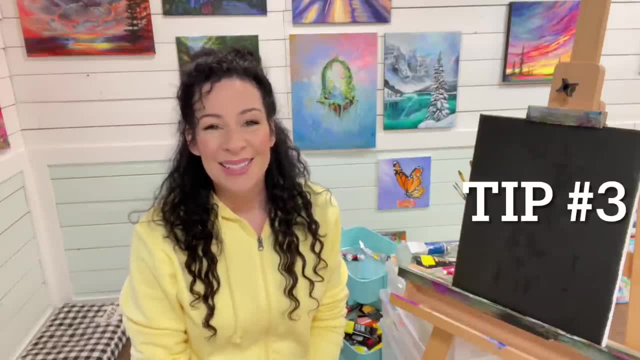 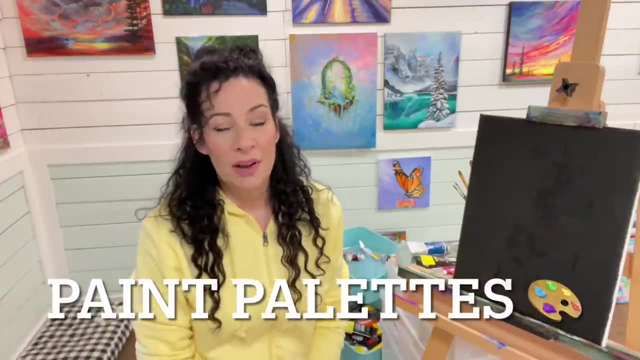 fridge and they'll stay nice and wet for you. and let's go right into tip number three now, choosing a paint palette. so there's a few different options here for you. I'm gonna start off with the one that I made the video for, and, if you 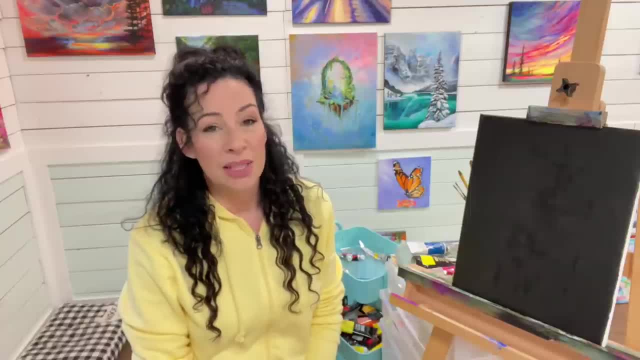 guys don't know already, I'm a resin artist as well. I love to work with resin. I make a lot of different resin things. I pour resin over my finished painting sometimes and I make all sorts of resin projects and art pieces. so I discovered that they make wonderful paint. 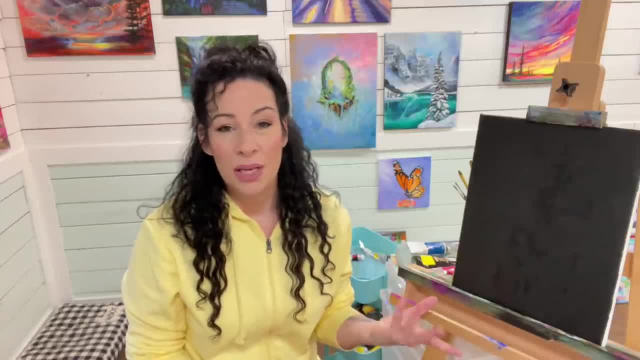 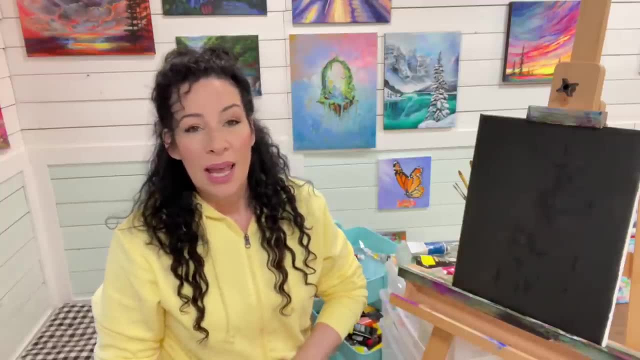 paint, paint. so you can just take any canvas that you want. you can even do like a really pretty under painting. I did some swirly abstracts and I threw in some glitter and I poured the resin over it and it's very smooth and waterproof and 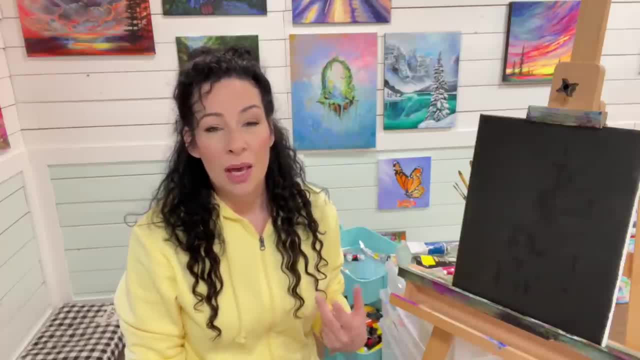 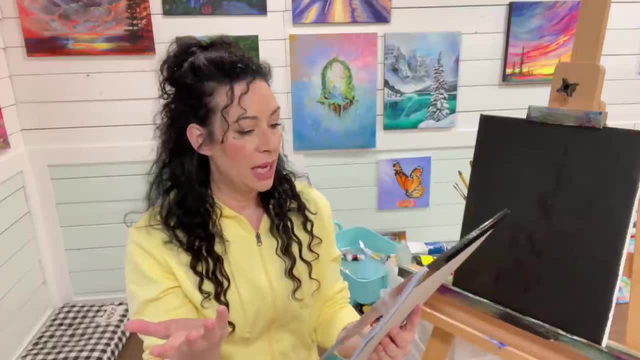 slick, so it works wonderful as a paint palette, but what I really like to use right now are Arteza paper palettes. I'm not affiliated with them, I don't have a discount or anything, but I'm gonna leave a link below for sure for you guys. this is something I just ordered these off of. 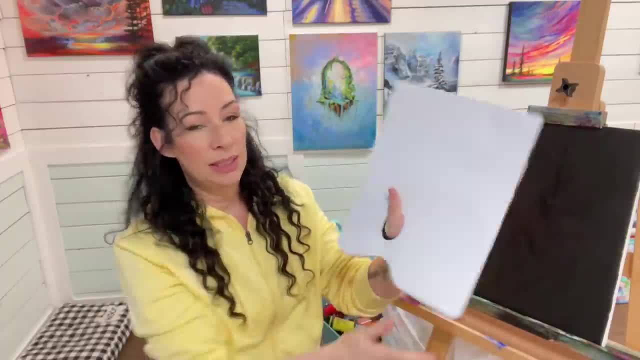 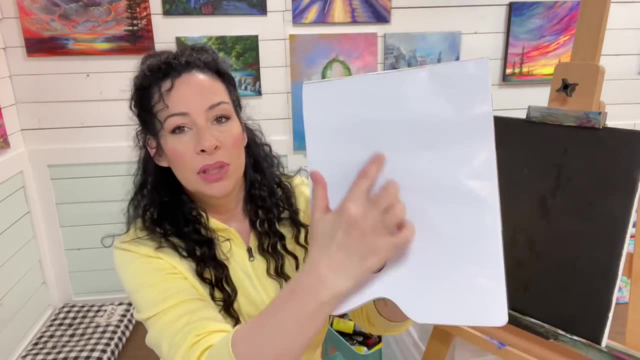 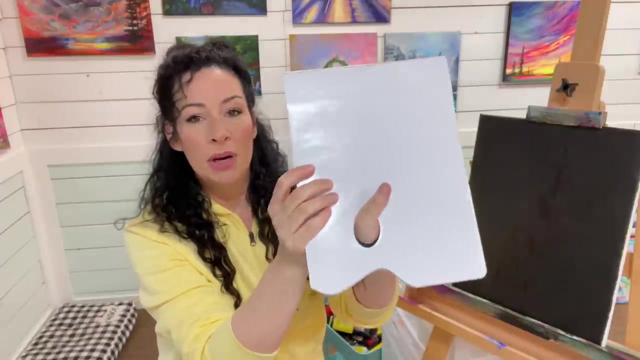 Amazon, and so I really like it because it's in the shape of that traditional palette, so you can hold it like this, put your thumb through and check this out, guys. so it's a really slick surface. it's kind of like plasticky, or even like parchment paper or wax paper, so these can last a long time and you can even 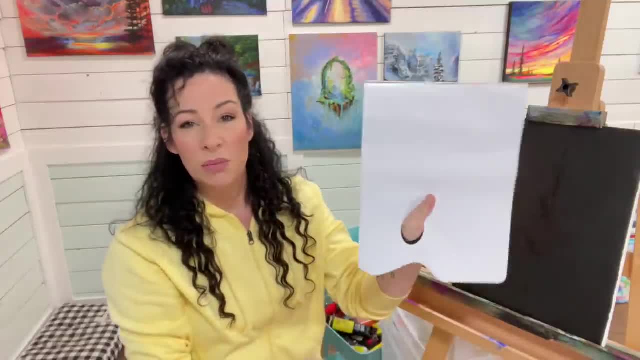 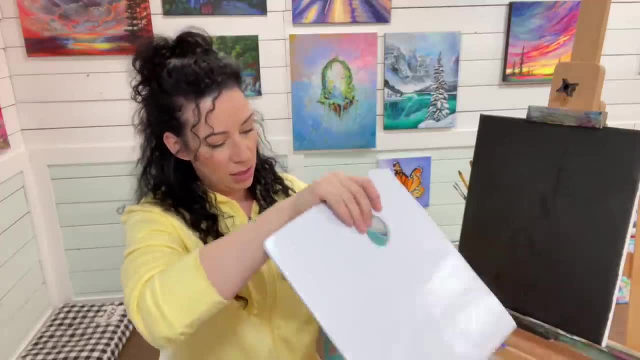 wipe them off. if you take the time, you can wipe the paint off and reuse them over and over, or you can just peel it off, throw it away. there's, I think, how many coming up. there's 40, 40 disposable sheets and they're quite big, so you can fit a lot of paint on there. 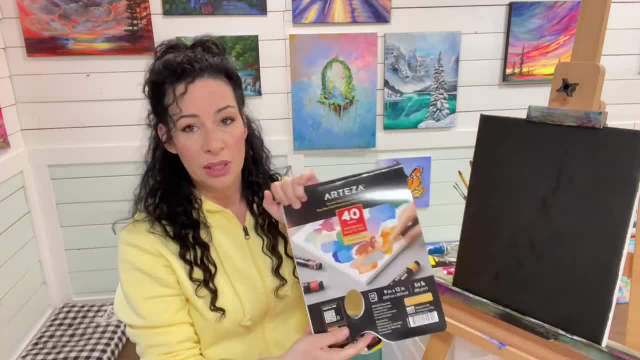 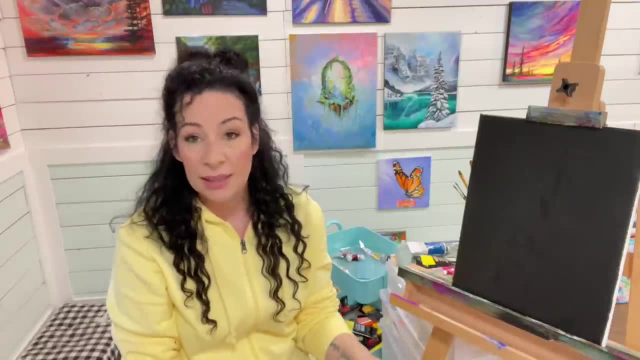 now if you and they're quite affordable too, I think they're. this is all under $20 for, depending on where you live and where you're ordering from. so, that being said, it's like it's very similar to wax paper or parchment paper, so you can. 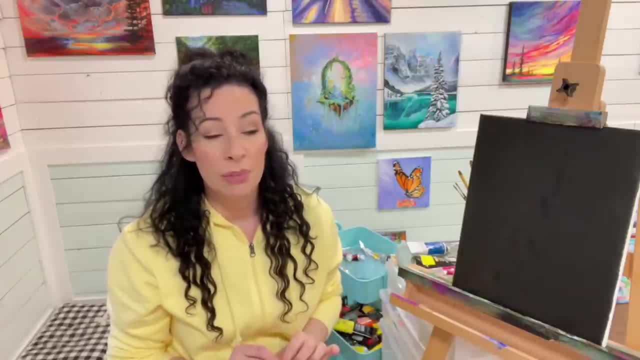 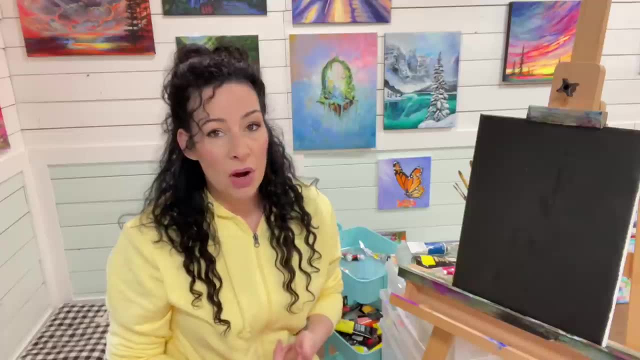 definitely use that. you can tape down some parchment paper, wax paper to an old cutting board or a piece of cardboard- and speaking of cardboard, you don't the. what you don't want to use for a palette is anything that's going to be absorbent, so you don't want, or porous, so you don't want to use any paper paper. 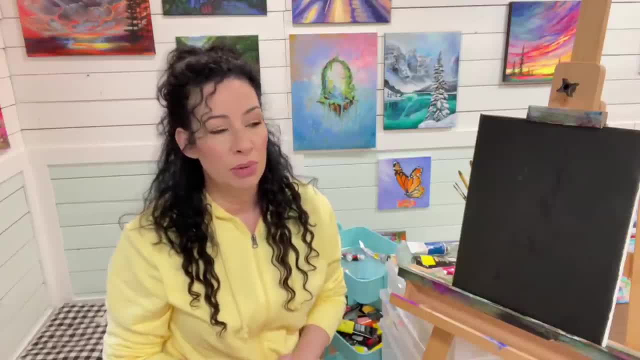 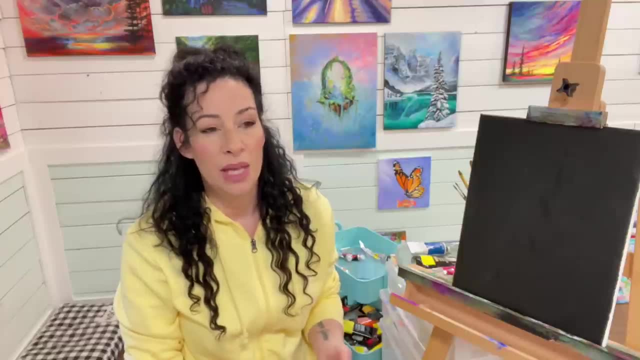 plates. I know I see so many beginning artists using paper plates and it's so frustrating because it just takes all that paint. so you're losing your paint. you can't, you feel like you can't keep up with it and yeah, so it's all the paint up, so you want something that's waterproof. 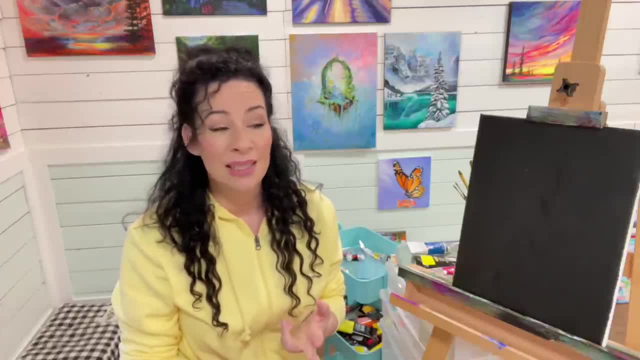 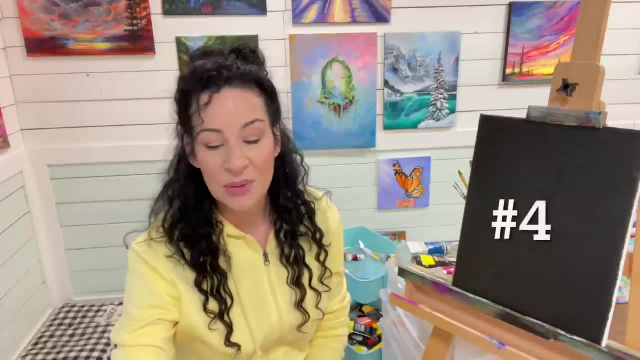 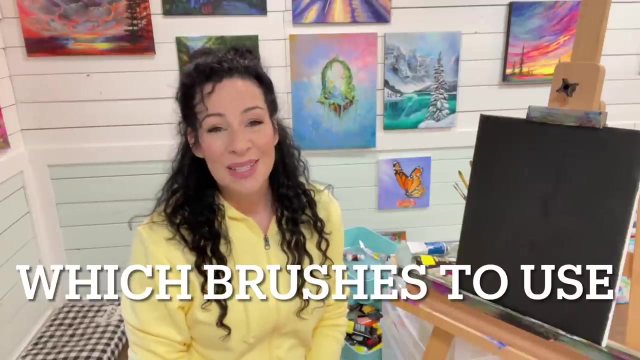 and wax, paper, plastic lids. you can get so many things from dollar stores, cheap things. so anything plasticky like that will work okay. so now we're on to tip number four. so for tip number four, it's brushes, and I've got another video I did a while back of my top five. just I think it turned into six of my must-have. 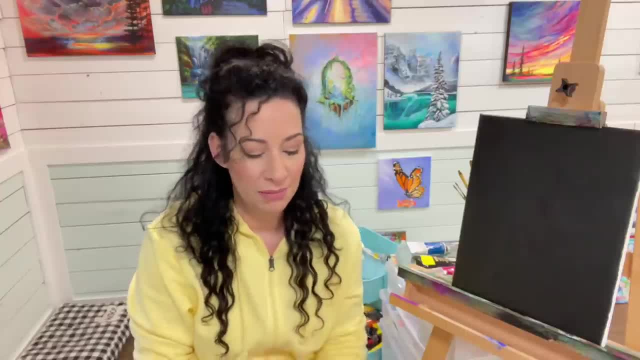 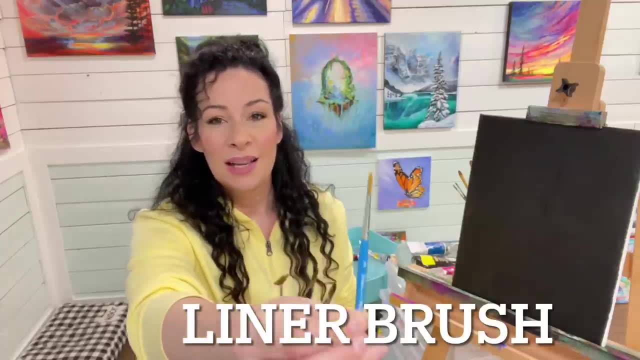 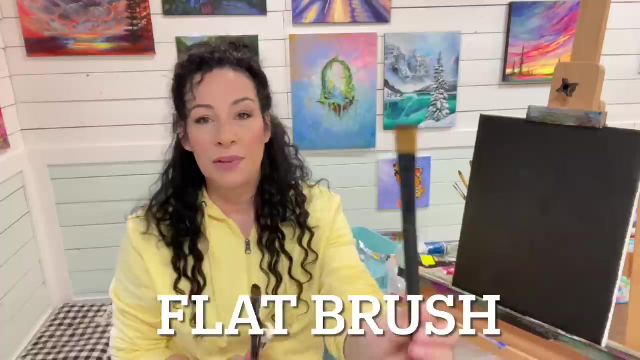 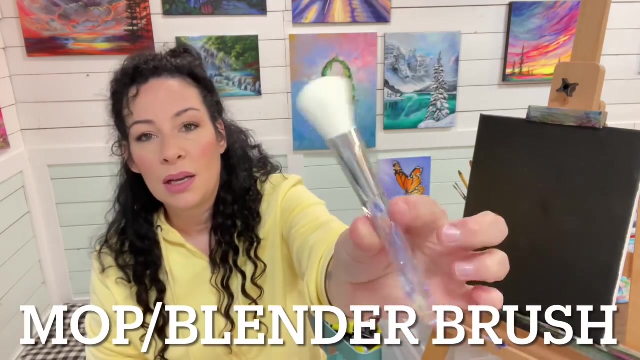 brushes and it hasn't changed. I've experimented with a few other brushes that I have. here is, or are, a liner brush, a fan brush. you're definitely going to want a fan brush, a flat brush. also got a filbert brush and a mop brush, or some artists call it a blending brush. so you'll notice this may look like a. 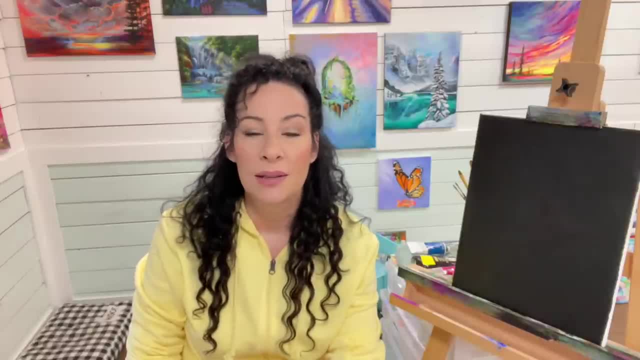 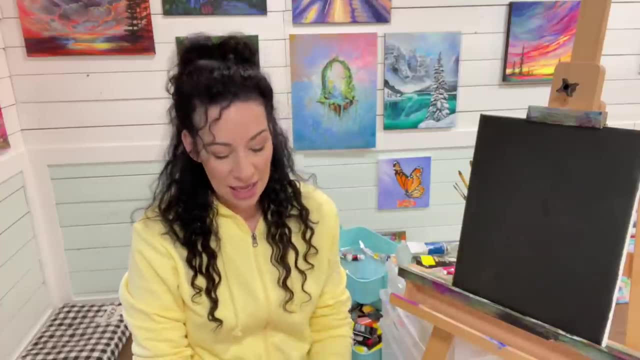 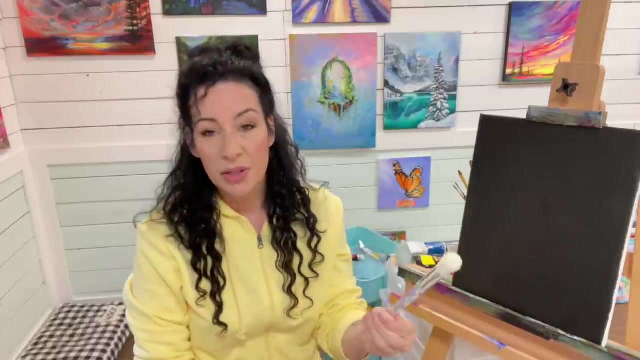 makeup brush it is. I discovered that I love using makeup brushes- blending brushes- for um all of my foliage and trees. so the reason why, and specifically these ones- i have a whole bunch of these. i recommend getting all these brushes in a few different sizes, so you want. 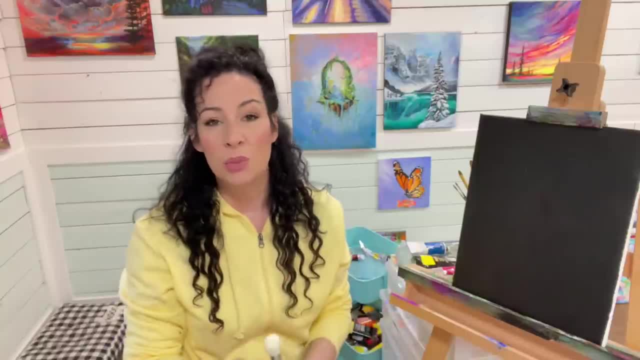 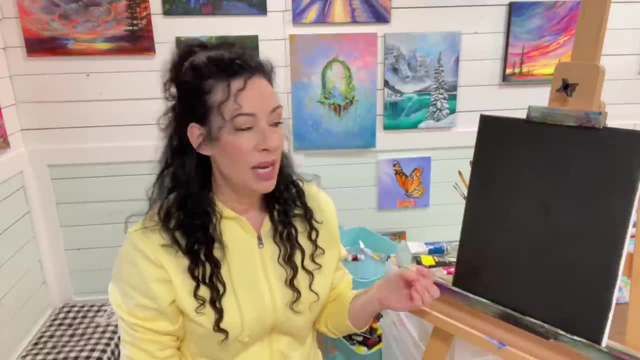 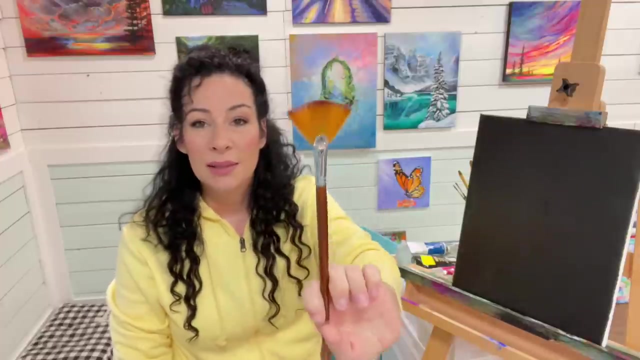 to have at least two to three, and your collection will grow over time. but we're always working on different sizes of canvas and subjects in our painting, right? so sometimes you're going to paint a big tree, so you're going to need, you know, for a big tree on a big canvas, a large fan brush. but if 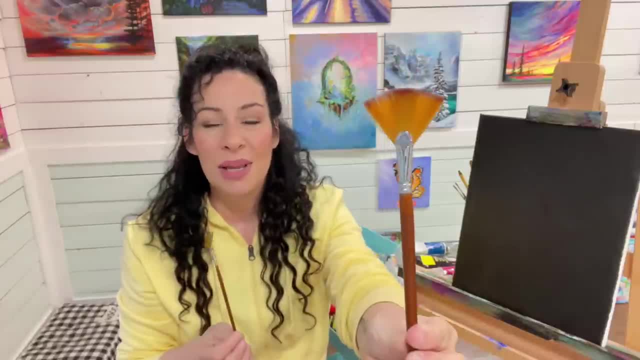 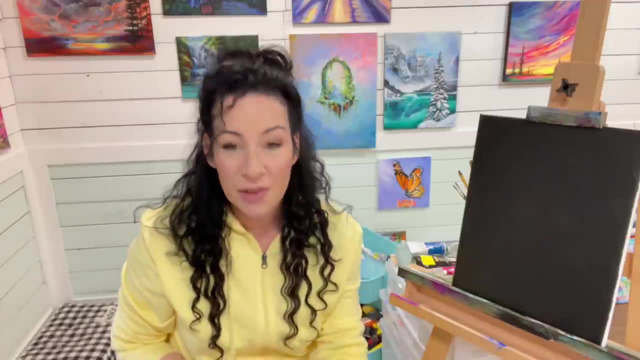 you're going to be working on a smaller tree. it's going to be hard to paint a very small tree with a big fan brush like this, right, so you make sure that you have some small ones. um same with a filbert. i've i've got 10 or so different size bilbert brushes and again it comes over time. 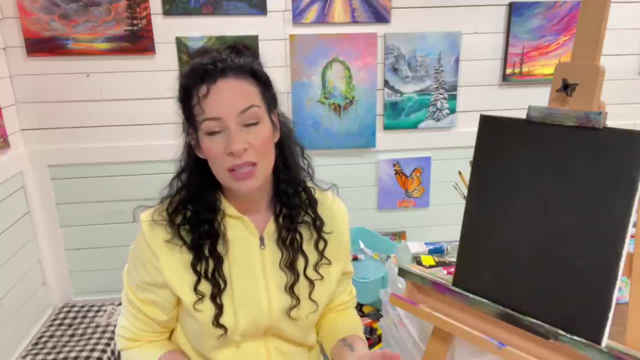 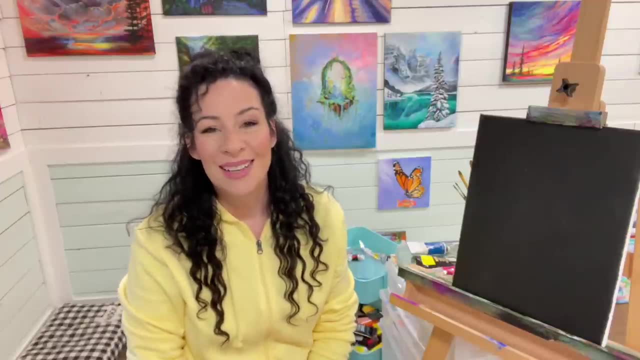 it's expensive at first to go and buy all that supplies. maybe just stick to um two different sizes, a large and a small. for now i'm going to go with a big tree, so you're going to need you know, until you can um acquire more sizes in your collection. but back to the makeup brushes. i 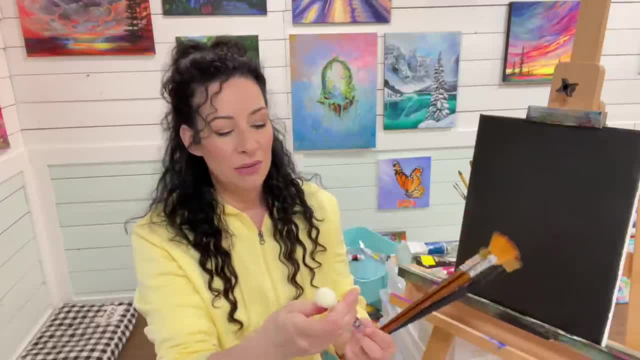 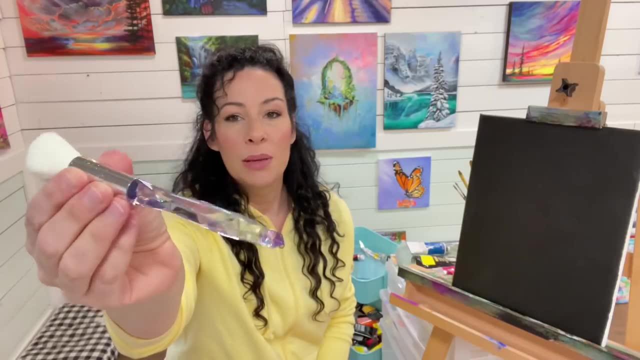 like these because um and i've been getting these on amazon for a few years now. first of all, because i like pretty things. it's iridescent and it's like all those pastel rainbowy colors in there. i love it. it's so pretty. that's, to be honest, what really um made me want to buy them, and 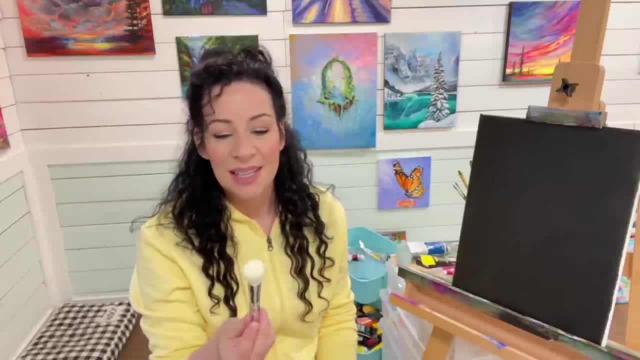 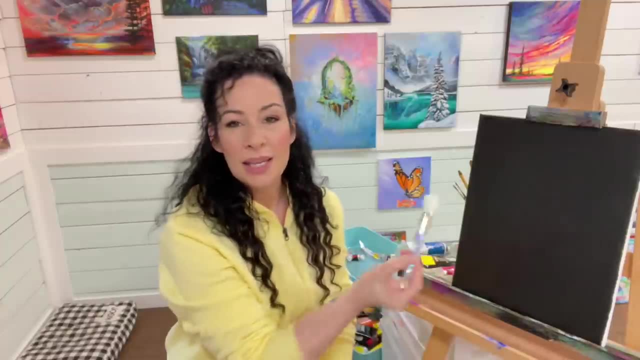 i bought them as makeup brushes first, so i tried one of these and it was amazing. it's so soft, but it's not too soft. it's just got enough give to it that i can. it makes the perfect. it's so satisfying to use and it makes the perfect little bushes and foliage. 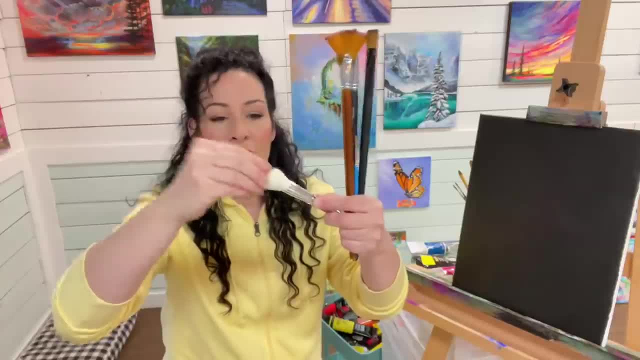 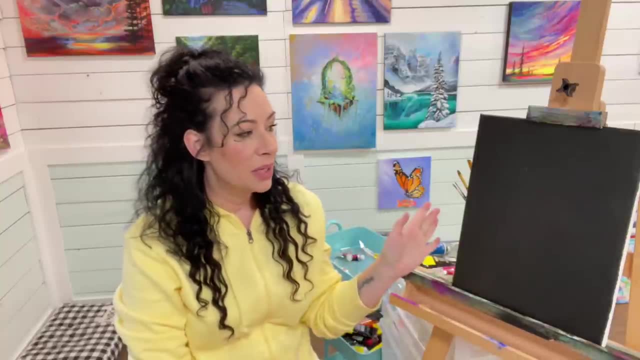 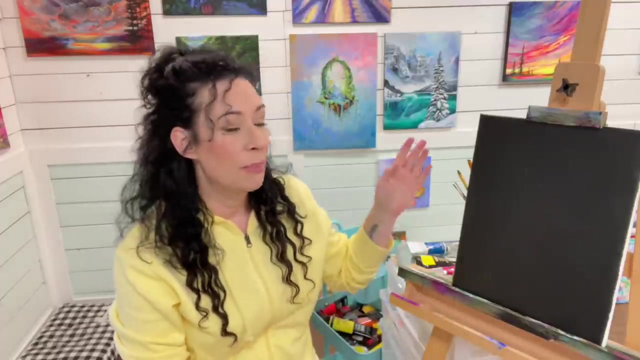 and another huge plus is that i haven't lost a hair to these. i mean, i've been using these for months and months and there's no hairs that are coming out. i will be demonstrating all these brushes for you guys in that other video that i've linked. below this one, you can see a painting. 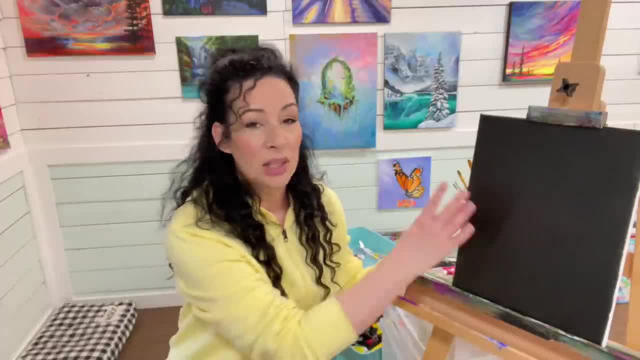 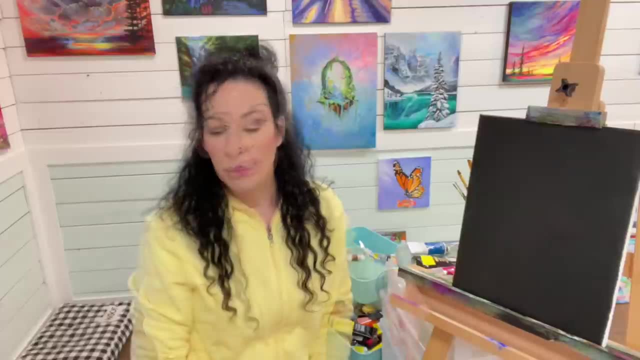 tutorial from start to finish with all my must-have brushes, slowly breaking it down step by step for you so you can see exactly how i use them, why i use them and why you guys should use them too. when choosing paint brushes, it can be very personal and individual. all of mine are different. i to be. 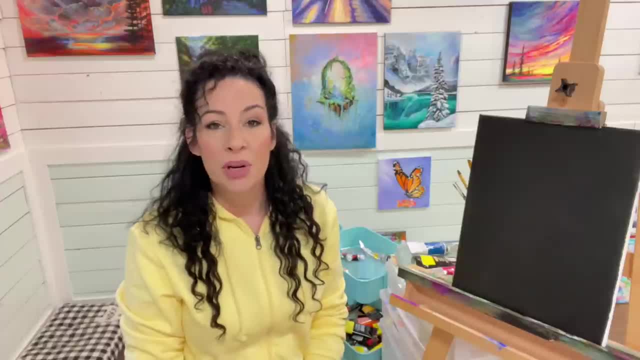 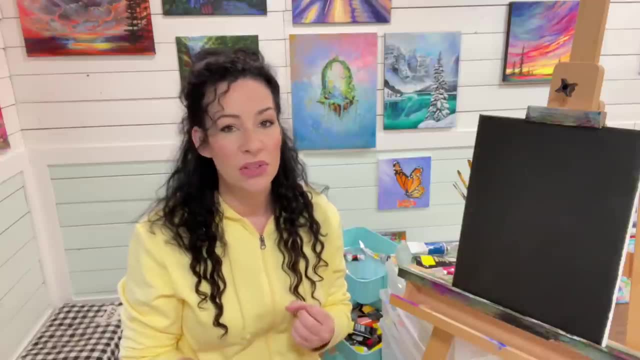 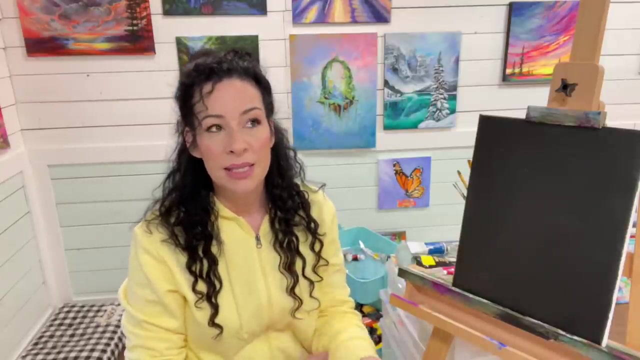 honest, never really look at the type of bristles when i'm choosing a brush. i just kind of feel it, kind of tap it, and i know the stiffness or softness that i that i want. um, i like how the will feel in my hand. so i'm not really going to recommend any specific bristles for you guys. 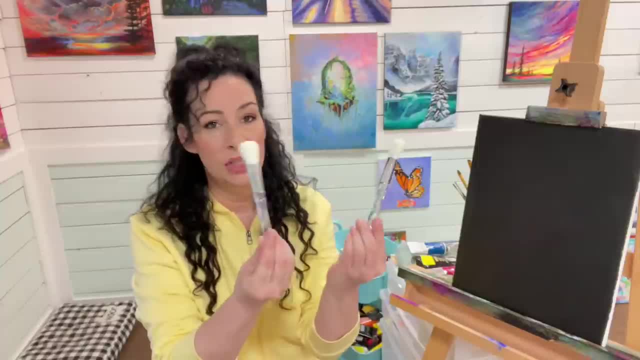 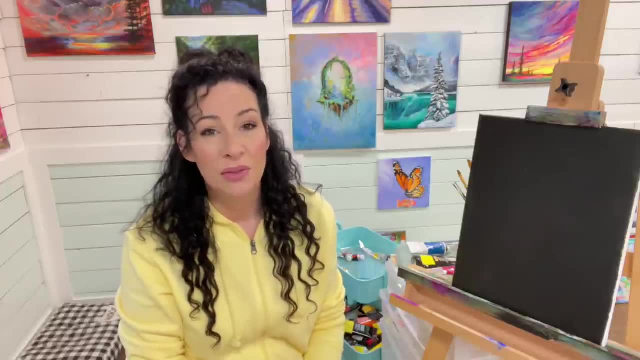 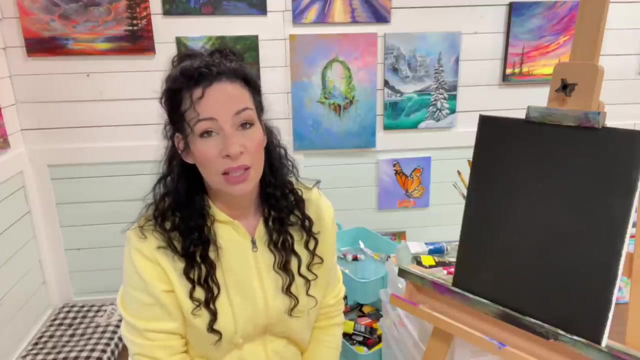 or brushes, except for these ones, because these are just amazing. um other than that, it's really personal. i recommend just experimenting yourselves and finding the ones that work best for you. um, so there are some that are really expensive. you don't necessarily need to spend a lot of money to get a good brush. tip number five under painting. so you can see, here i'm 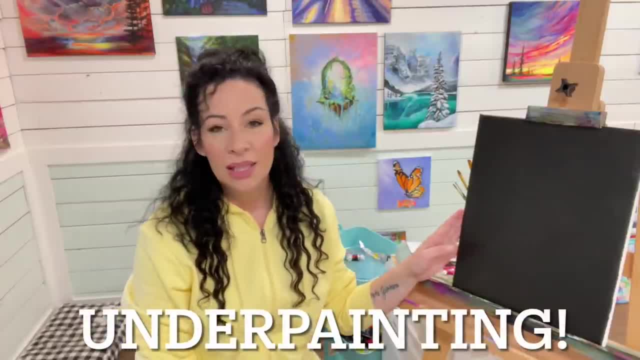 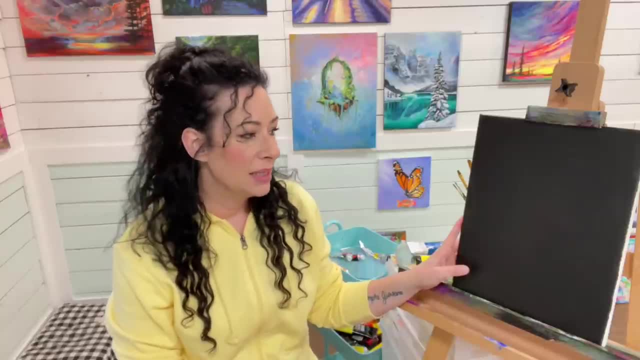 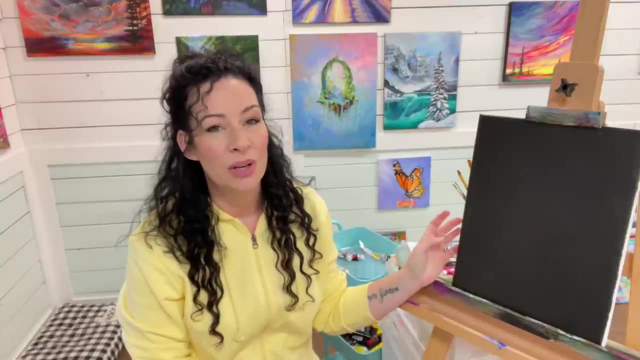 i've got a black canvas. i really love painting on a black canvas. i like painting on white canvases too and a few other colors, but black to me is very exciting. i love the way the colors pop off the canvas. i love the instant shadow and contrast that i get from this, and you know, to be honest. 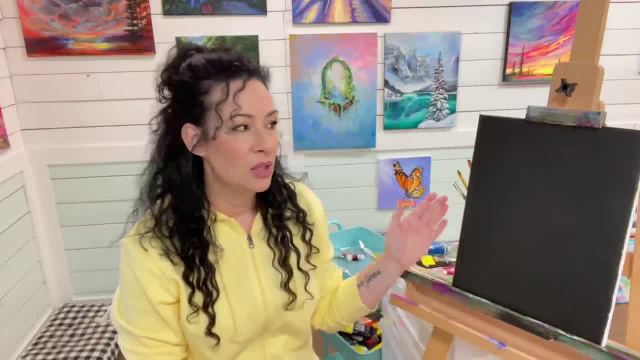 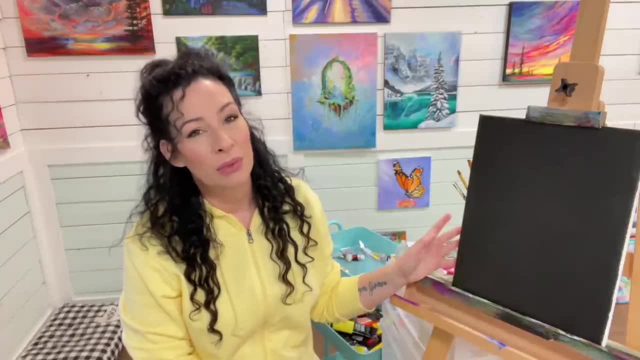 it's a really quick and easy way to cover up an old painting, so usually just need one coat of black because it's so strong. if you take white paint to cover up an old painting, you're going to take like three, sometimes even four coats of paint to cover it up. but if you 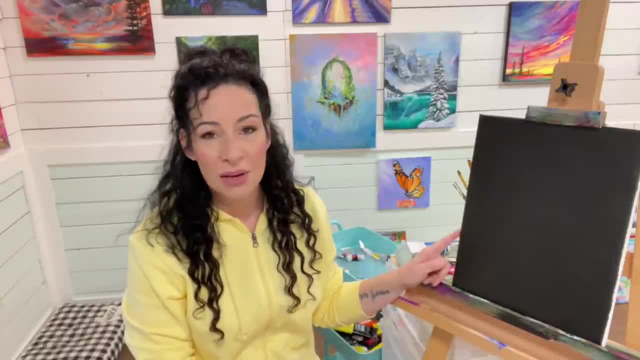 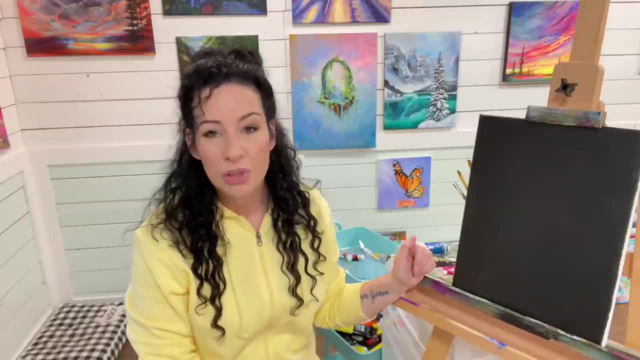 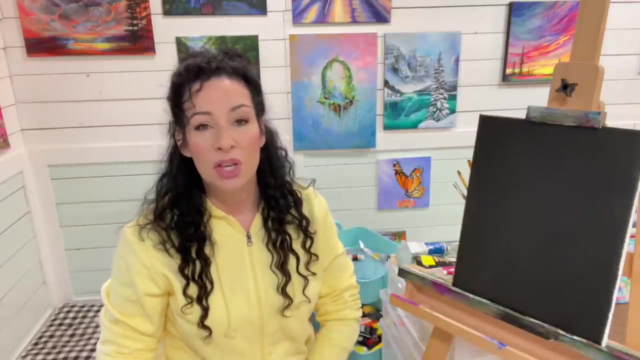 just take black. it's a lot easier. so that's another big reason and tip why i like to use black paint to cover up a canvas with um. there's other options. you can use black gesso. i think i touched over a few things about gesso at the beginning. there's different colors of gesso. you 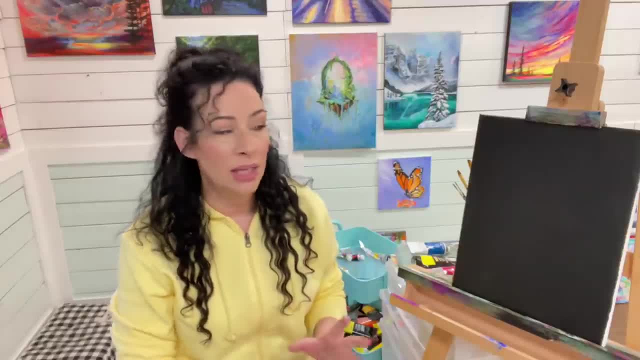 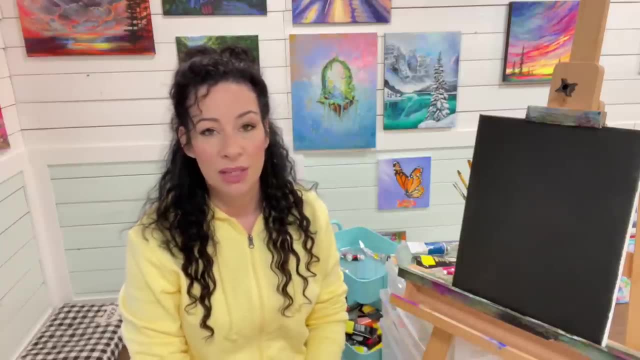 can use. um, if you want to do two in one, you know, kind of just get it all done, the gesso and your under painting, then that's something to think about. if you're just going to paint the canvas about, then you can, you know, skip a step. you're getting two things done at once. 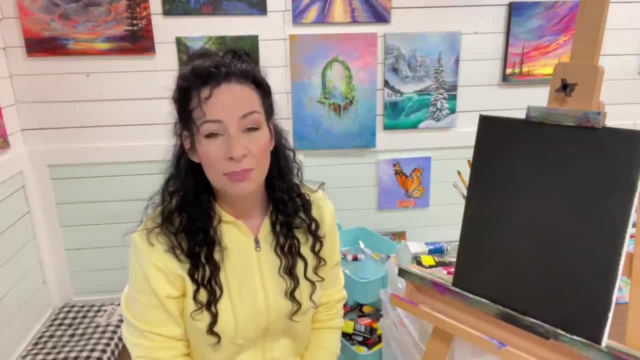 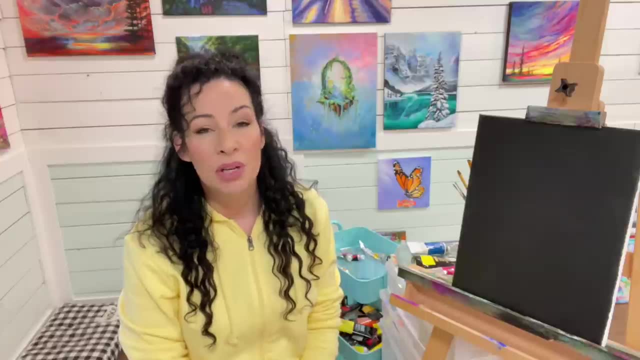 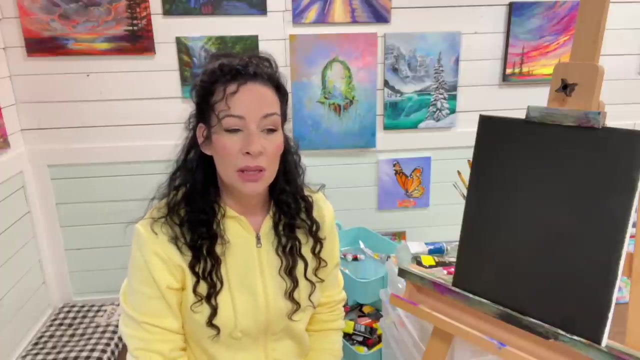 there's other colors to consider. under painting, a lot of artists like to use warm, rich tones: oranges, yellow, ochre, burnt sienna, burnt umber. um, i love a bright, bright red. i kind of like to think about the main color. if i'm doing a painting that's going to have a lot. 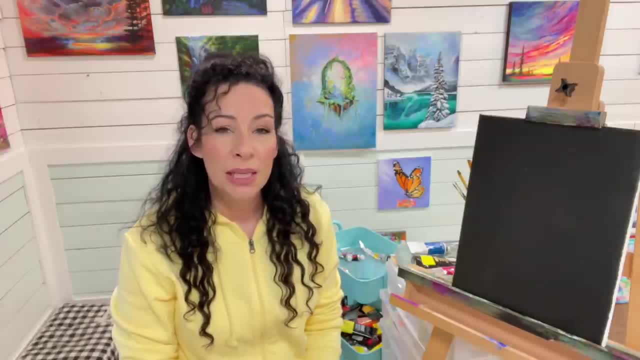 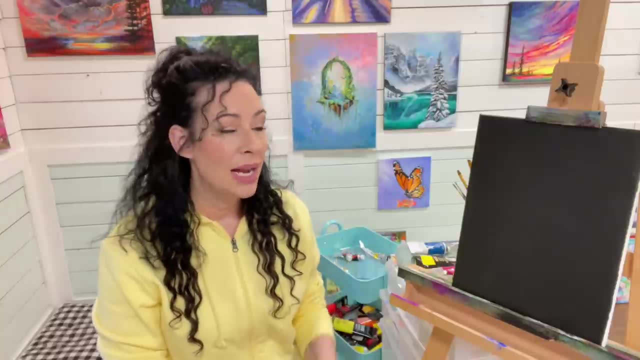 of green in it, let's say a forest painting, something that's going to have a lot of green trees in it- then i like to think and look at the color wheel for the complementary color of that. i know that if i work on a red canvas, any shade of red it doesn't matter, you can use bright. 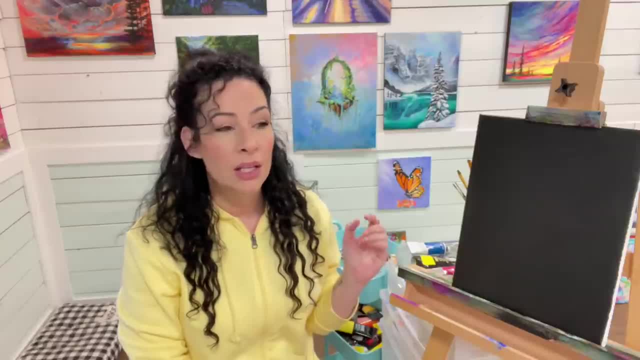 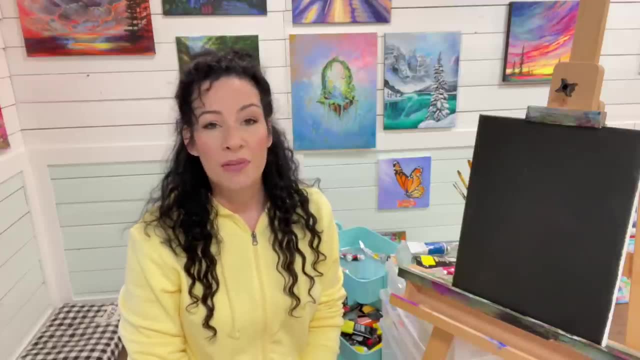 bright, neon red. you can use a dark red, no matter what red it is. it's going to make your landscape or whatever you're painting stand out even more. it's just going to pop off the canvas. it's just kind of like a magical little thing that happens. can't explain it. the colors really like each other. 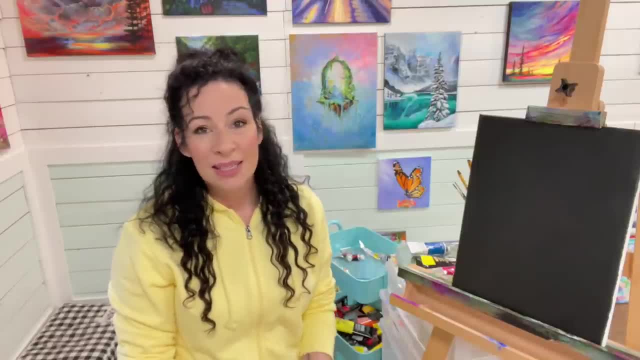 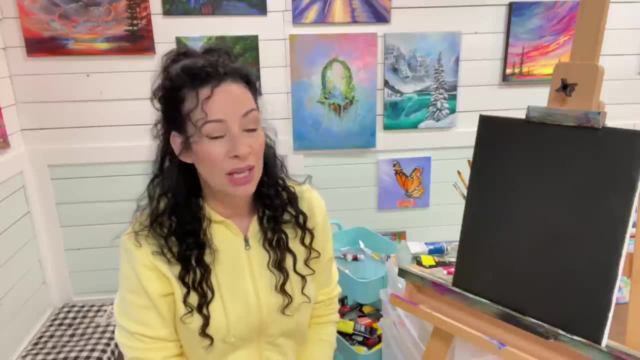 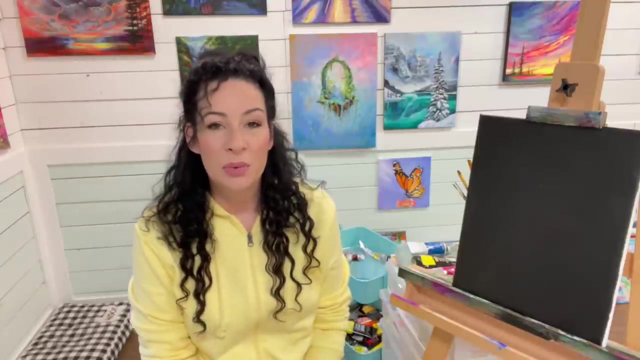 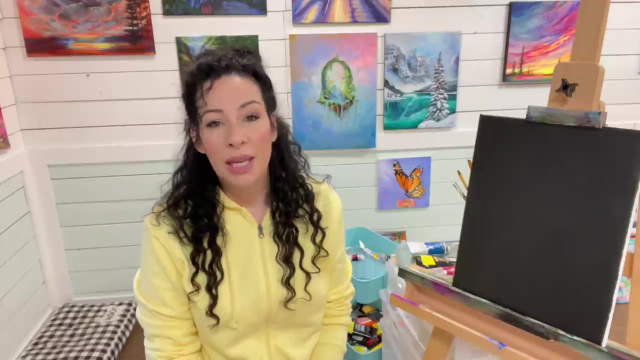 and i love how it kind of makes the canvas more vibrant and more vivid and more vibrant. so i'm going to take a few more colors and i'm going to go ahead and start with my. this is a nice color that i like using for my canvas, but i do use some other colors, but i'm 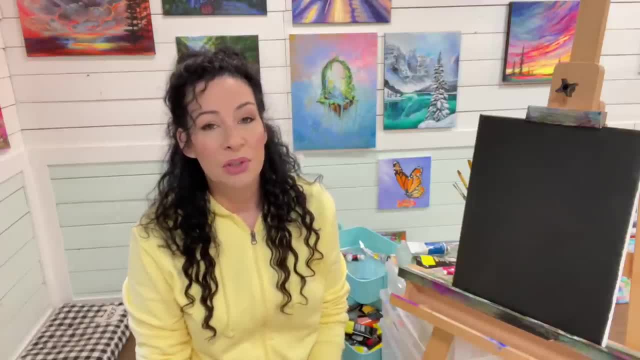 definitely going to take a few more colors and i'll just show you how that looks like. i'm going to take this one and i'm just going to go ahead, and i'm going to go ahead and i'll just. sometimes you can get the paint out of your clothes. I want to make sure that. 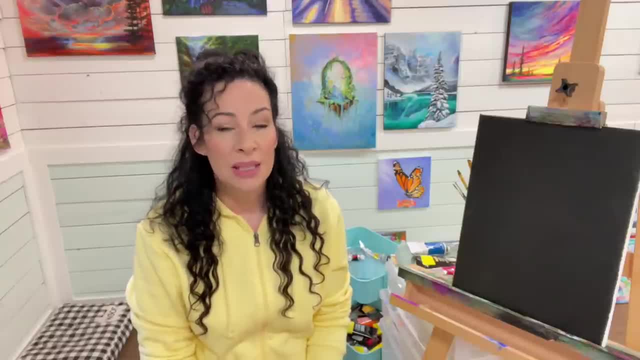 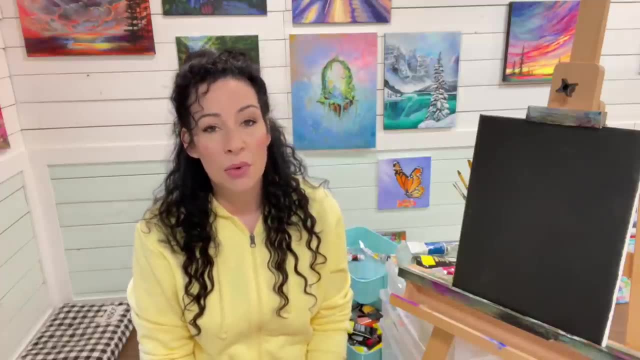 you're washing your brushes out, don't leave them sitting in water too long either. if you have your water, your brushes in the water too long, that's gonna kind of work: the handles, the paint is gonna peel off. it's gonna work the shape a little bit. it'll make the bristles and the brush start to rot and 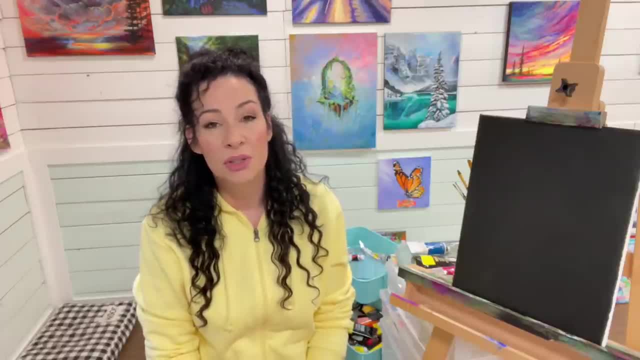 the bristles will start to come out, so it's not a good thing to leave them in water too long, and it's also not a good thing to leave your brushes out with paint on them. they're gonna dry, they're gonna be hard and stiff and you're gonna 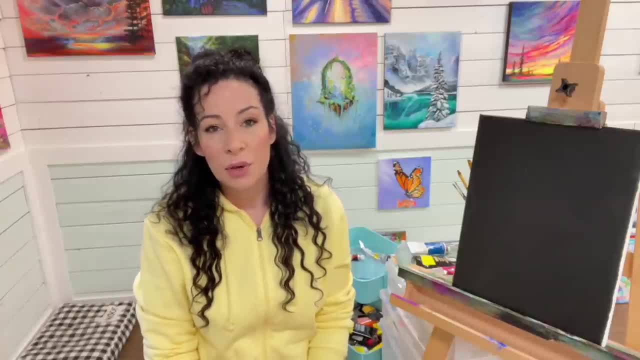 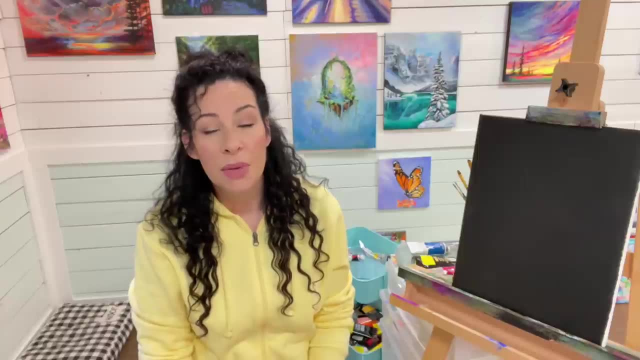 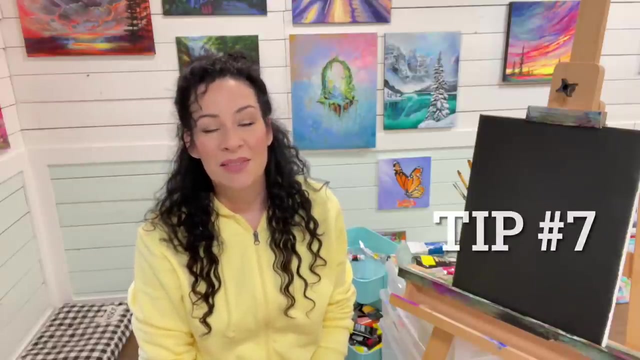 have to throw them away and at the end of your painting sessions, the final wash of your brushes, I like to do just a lukewarm water with a very, very mild silver detergent and then dry them off very carefully. okay, so for tip number seven. tip number seven today is: take advantage of the drying, quick drying. 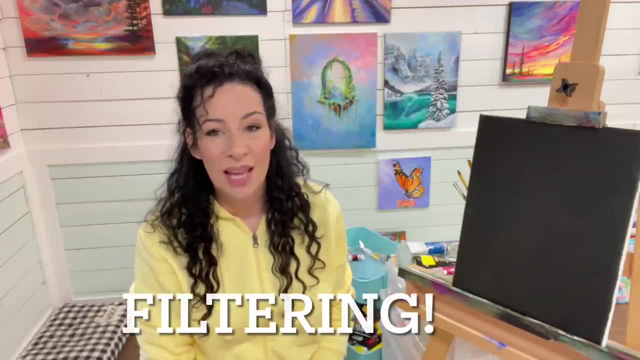 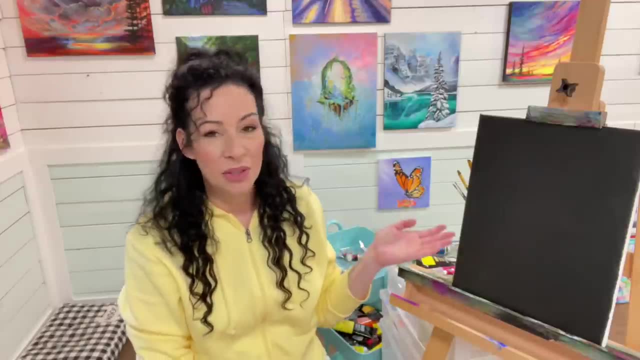 aspect of acrylics. acrylic paint dries so fast and so many people get frustrated with that, but I love it and I take advantage of it all the time. so what you can do is you can take advantage of the fact that you can do is apply filters over um your paint when it dries quickly, and this is really. 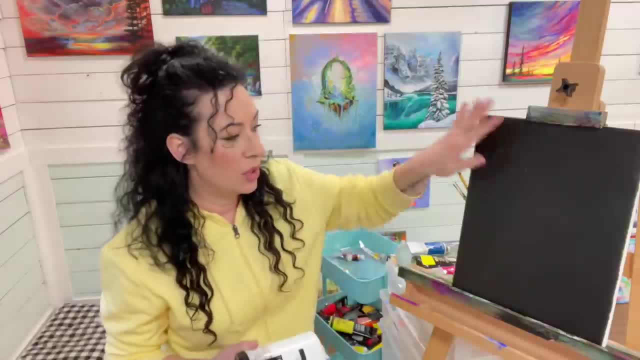 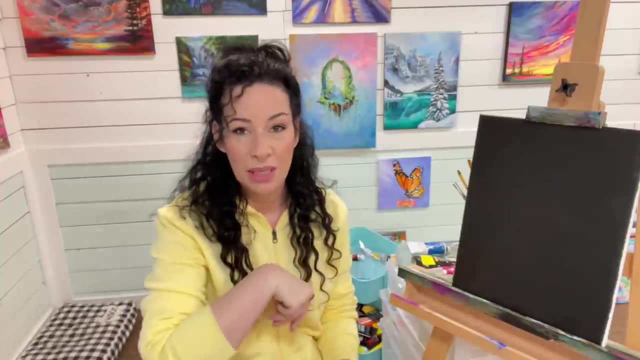 really fun to do. I'm going to demonstrate this right now for you guys. I'm just going to do a quick white wash over here and then I'll dry that off. so I'm going to speed this up and then you'll see what I mean about the layers. 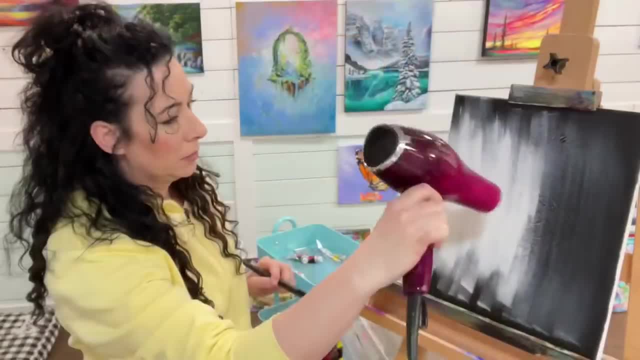 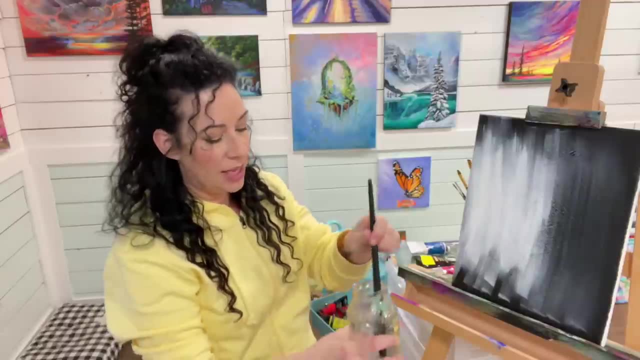 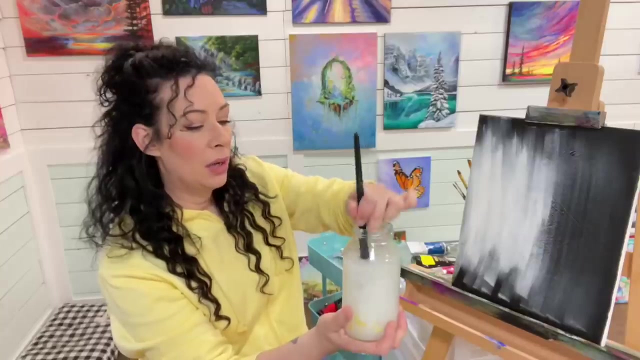 okay, guys. so I just painted a little bit of white on this canvas and I'm going to wash this paint out right away. so you're going to want to have quite a bit of water. I usually have a larger water jug here. I'm going to use a little bit of yellow. first. I'm gonna put the yellow here. 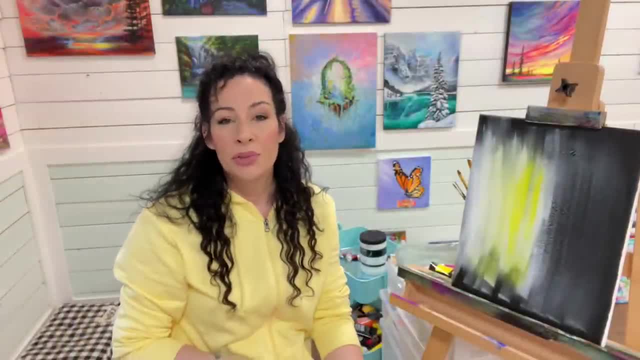 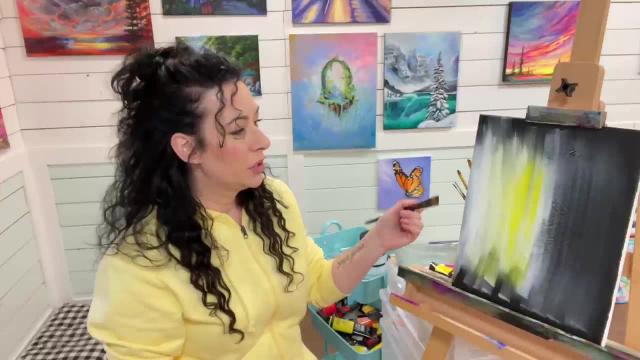 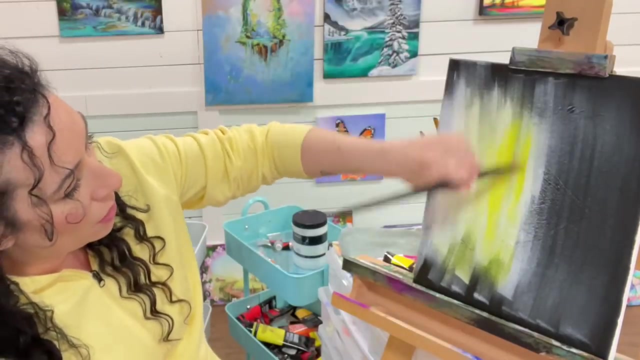 so what this does is it just helps you with skipping color mixing. if you don't want to make a specific color, you can sometimes do it, um, just right away, instantly, like this. so now I'm going to take some of my phthalo blue and I'm going to go over. I'm going to take 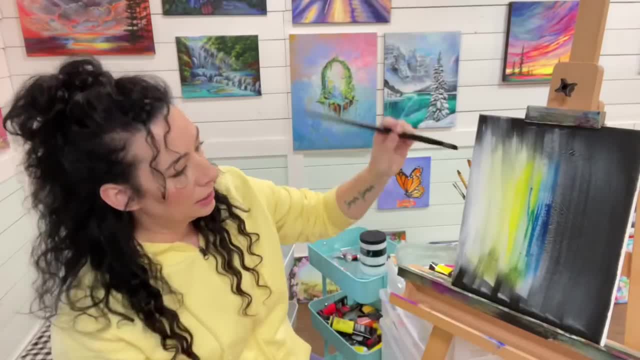 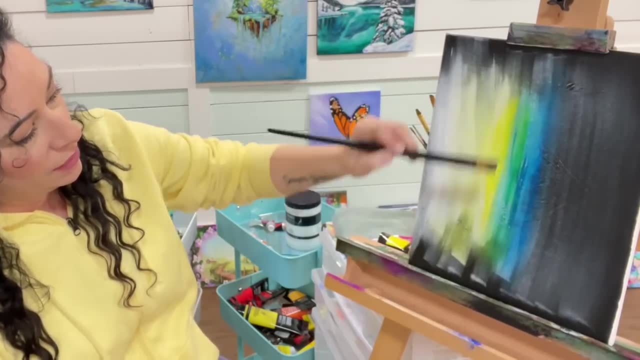 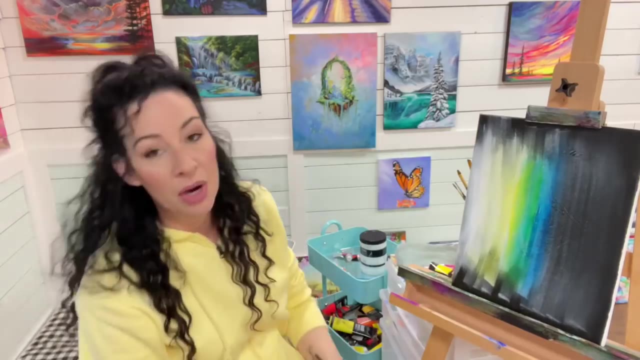 just a little bit of water, just a little bit like this, and I'm going to slightly go over part of that yellow so you can see my blue here, very beautiful phthalo blue, and then if I filter over part of that yellow then you get green right away. so that's what I mean with filters. it's 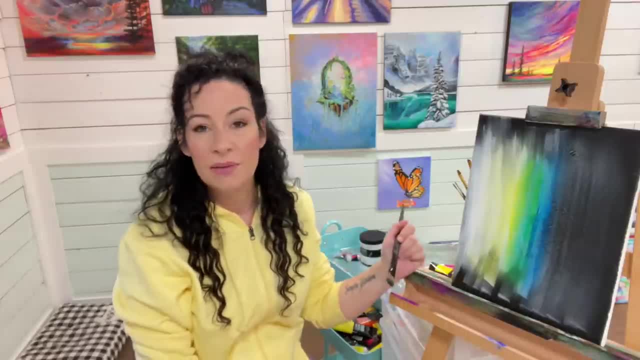 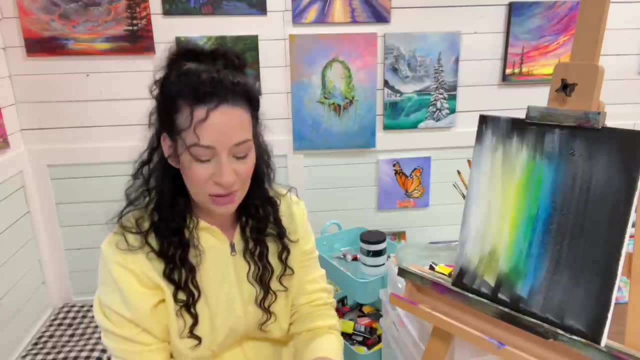 so fun and versatile. you can do so much with filtering and taking advantage of how quickly the acrylic paint dries. so I'm going to do one more example with uh, one of my neon colors. you guys, um are starting to really catch on with um, the joy of painting. 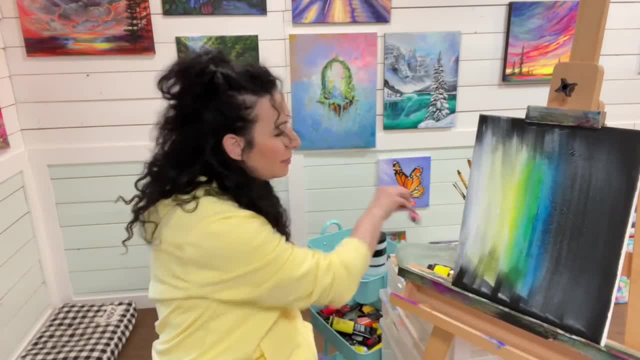 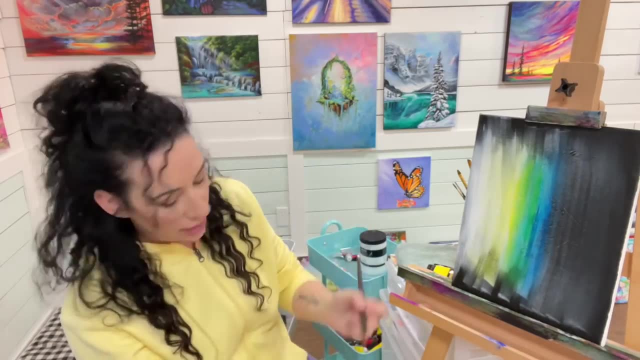 with neon colors. they're so, so much fun and for this example, I'm going to use my neon pink by Holbein just a little bit like this. I'm going to also take right away just a little bit of water and I'm going to start over here. 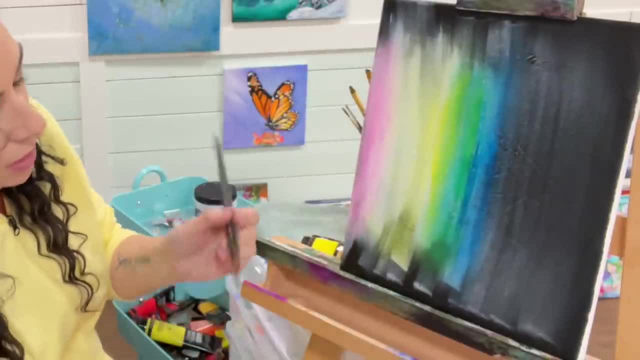 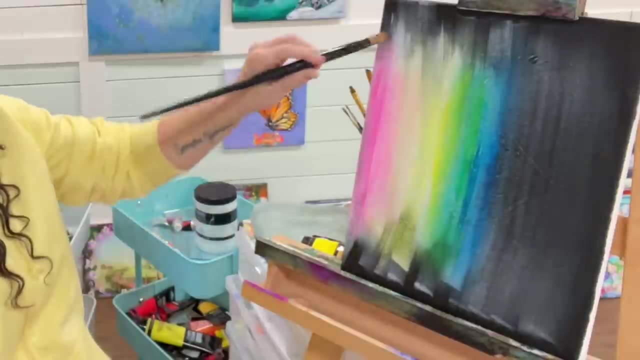 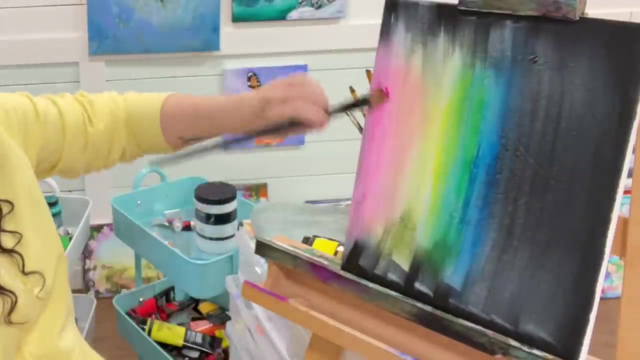 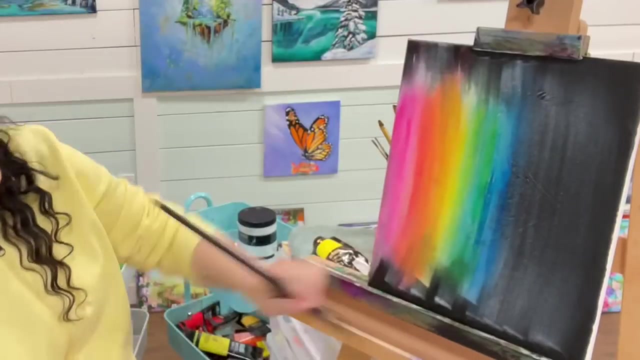 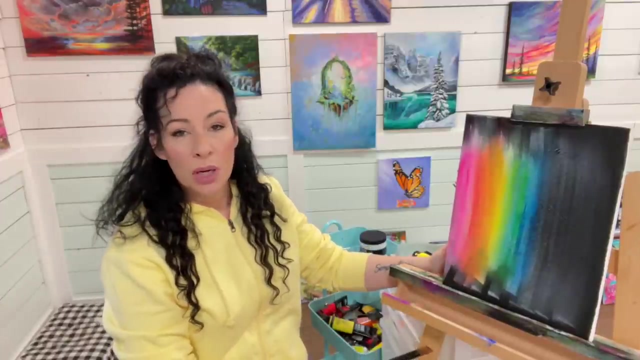 that's quite watered down. I'm just going to take a little bit more, okay, and then I'm going to work my way over to the yellow and, depending on how much yellow you have underneath, the more peachy or orange it's going to look okay. so there you can see, by layering, overlapping, filtering, whatever you want to call it- taking. 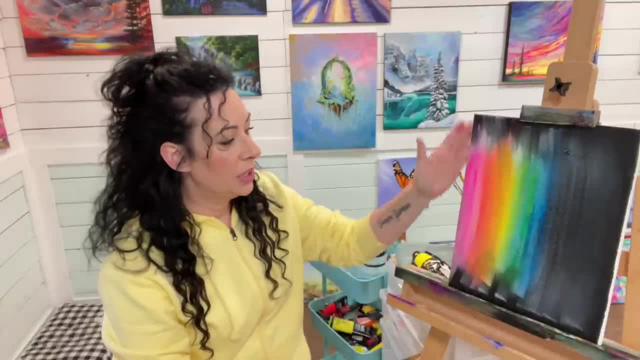 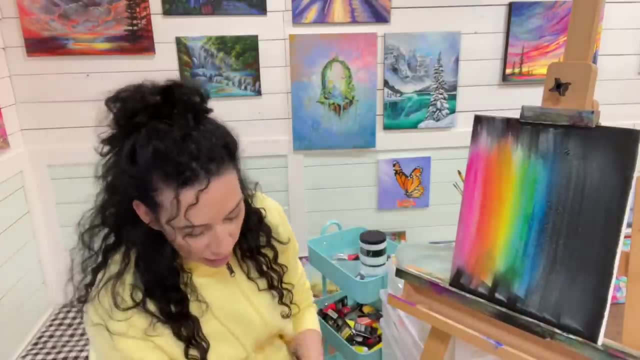 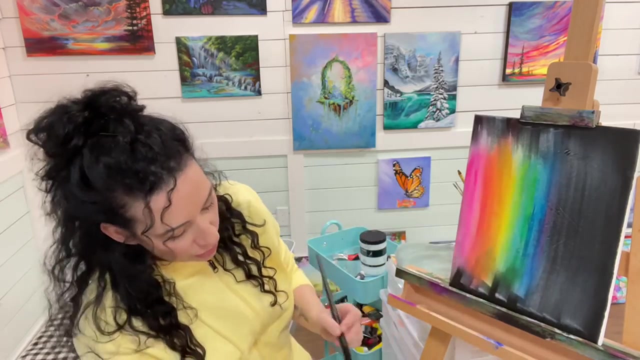 advantage of that quick drying aspect of the acrylics. you can create more colors instantly just by doing that on the canvas, and I can also make purple. if I take a little bit of the pink and go over the blue, of course, you'll get some purple. so look how many different colors that we've made. 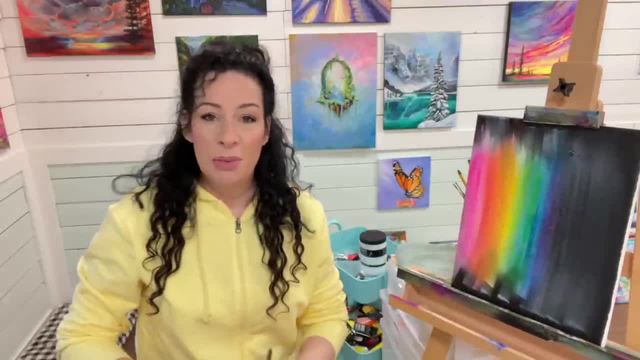 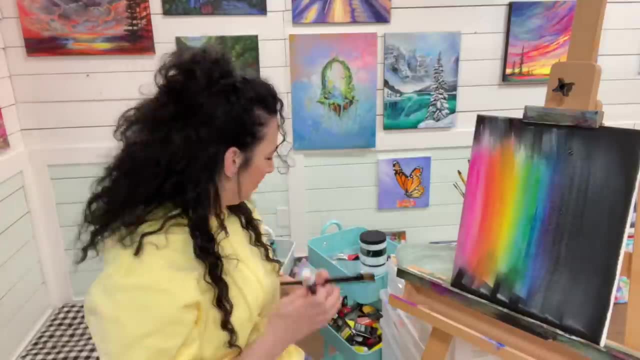 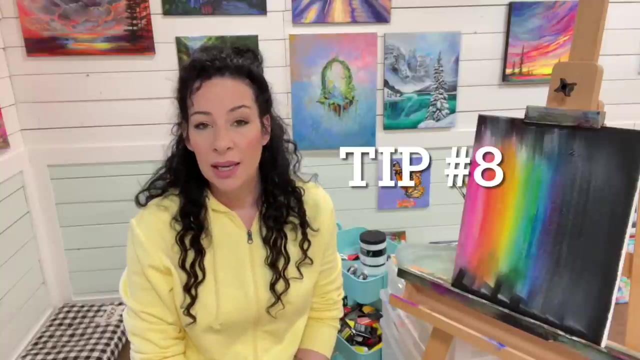 by layering over. so we pretty much made a rainbow just by layering colors over, like this with using blue, yellow and pink. and that brings me to number eight, next, actual color mixing. so if there's a color that you really like, oftentimes you can make it yourself. 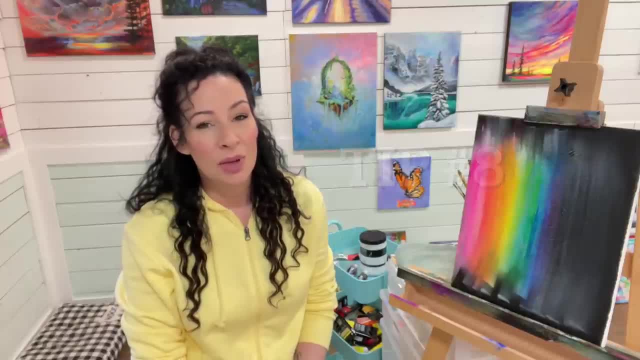 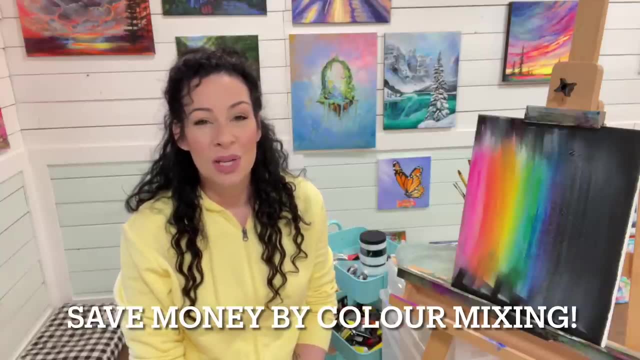 you don't need to go and buy that specific shade in a tube from the store. that will save you a lot of money. I've got a video that I'll link below for making turquoise and purple a very pretty shade of turquoise. different turquoises and purples below and in the future I'm going to be. 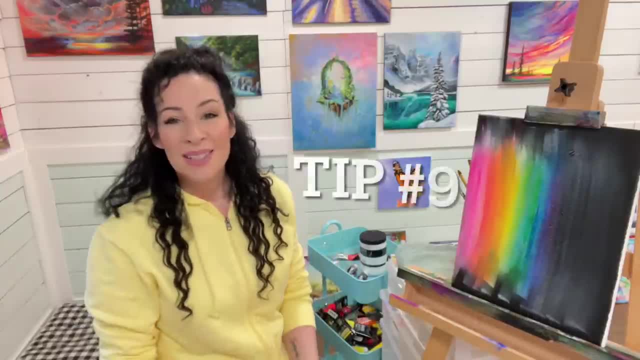 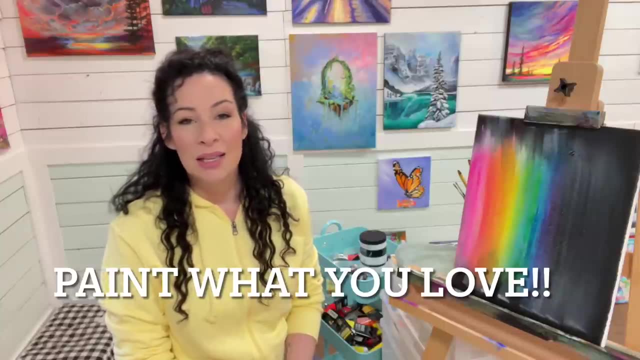 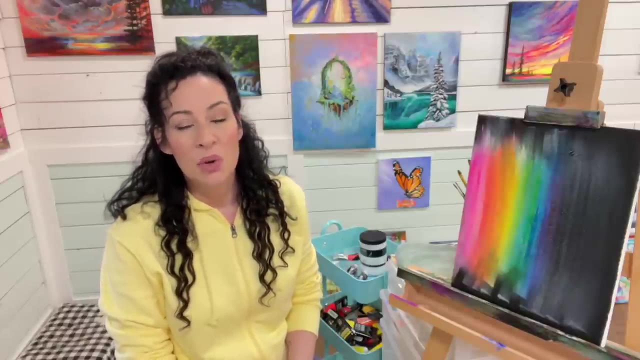 doing a more in-depth color mixing video. My number nine tip is: paint what you love. so I've given you the tools here that you need to paint successfully with. A lot about painting happily and well is by painting what you love. so I only paint things that bring me joy, and then I love to paint and I'm a. 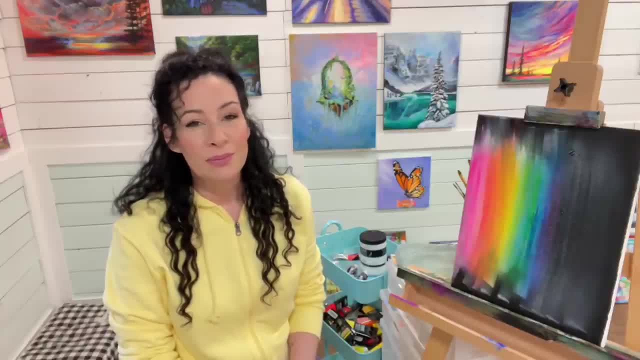 much happier artist because I started doing that years ago. If there's something that you're asked to do and you really want to do it, I'm going to be doing a more in-depth color mixing video. If you're really hesitant, because you're afraid you might not be good at it and you haven't tried, 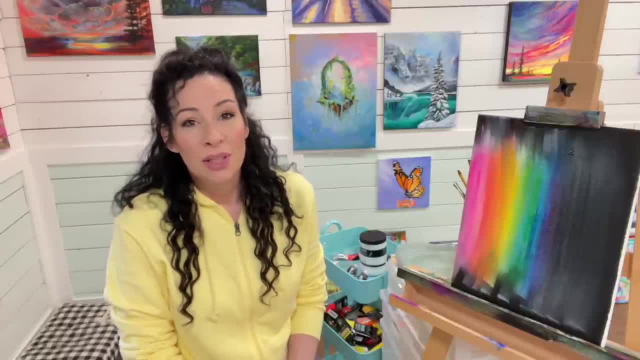 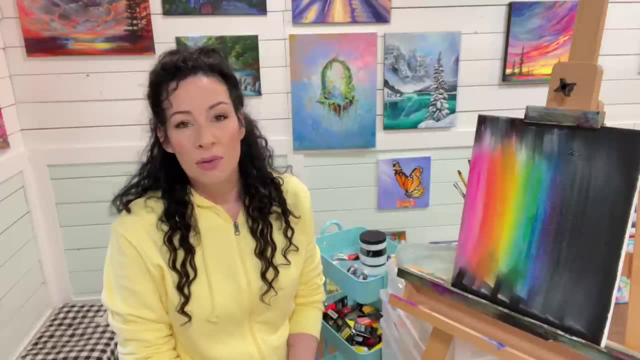 it before, then I do recommend trying it, because you don't know if you like something yet or not until you try it. If you try it a few times and you just really don't feel joyful while you're working on it, then I would recommend not painting that again. but you can learn a lot from getting 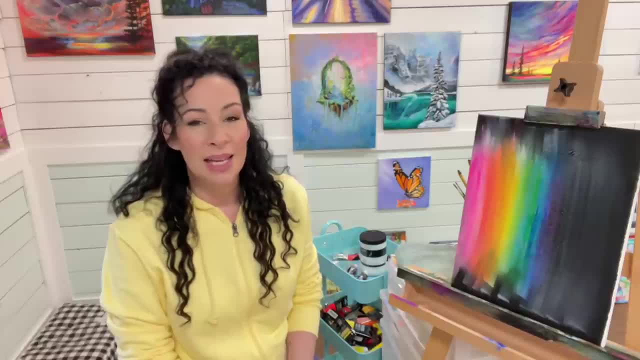 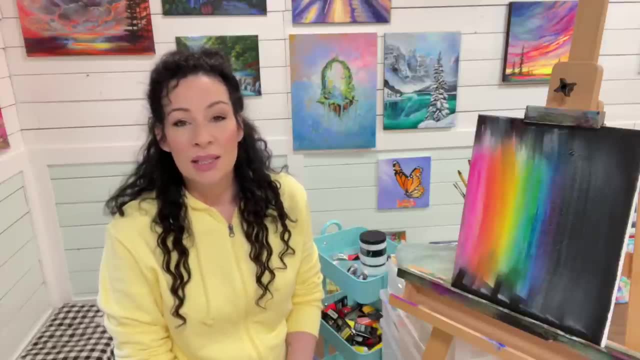 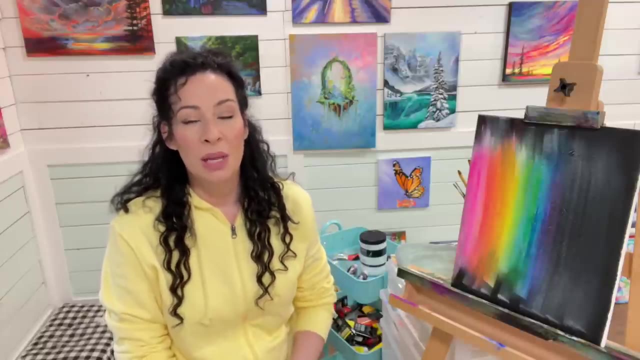 out of your comfort zone and trying to paint new subjects and landscapes and using different tips and techniques. So definitely try everything, but take what you can, you know, take what you learn from it, take what you can get from it and throw all of that in to what you love to paint, what brings you the most joy. Don't try to paint it. 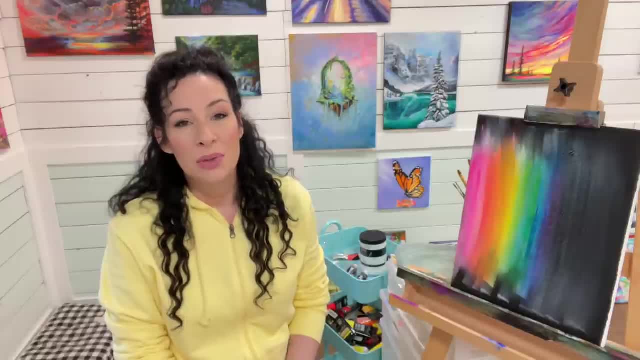 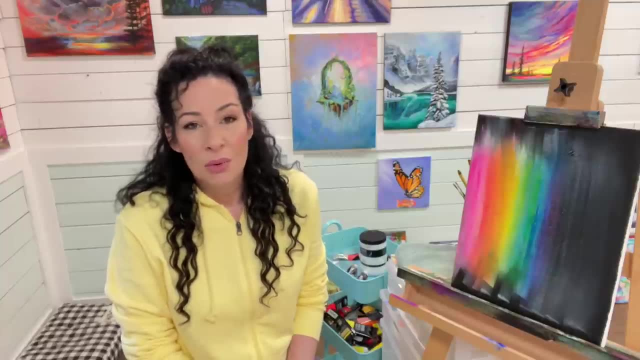 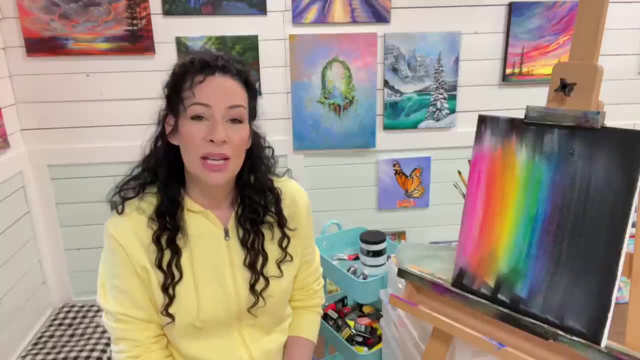 like another artist does. It's almost impossible to copy another artist's work, and we're not meant to do that. We're meant to express ourselves in our own authentic way. so that's what I like to do with my channel. I'd like to remind you guys that that's a big part of painting and creating. 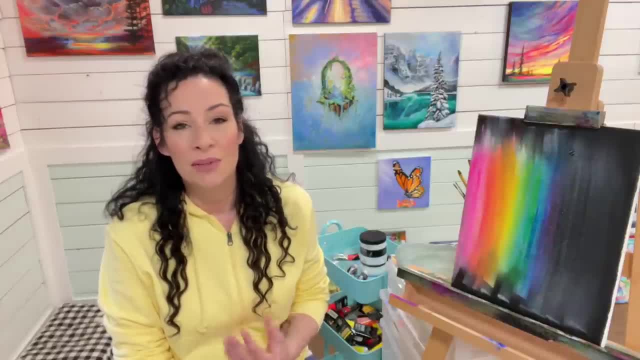 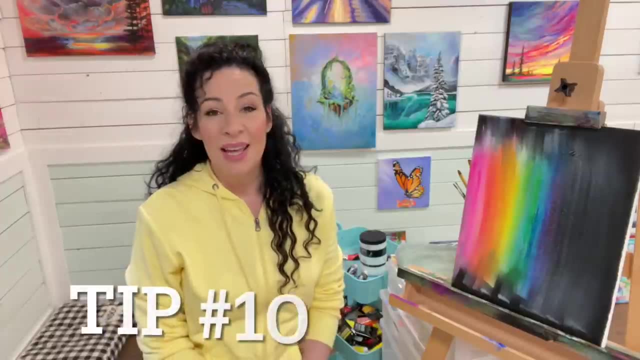 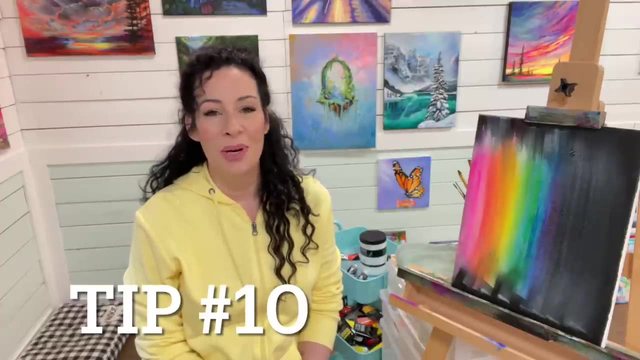 by delving into yourself, your inner self, your inner creativity, your authentic self help inspire you guys to express yourself in your own unique way. So my number 10, my final tip, is what to do when you're getting frustrated in a painting and it's nothing's working and you just want to throw. 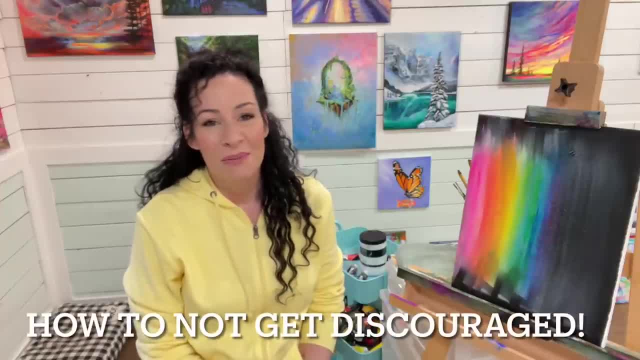 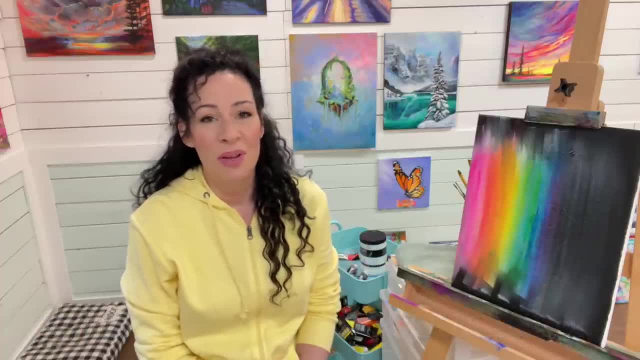 it out. We've all been there. I've been there before many times. uh, less and less as the years go by, because I've learned to paint more joyfully and to let go. that will come with time. it doesn't work that way, but for the majority of us, just starting out painting and really not knowing who, 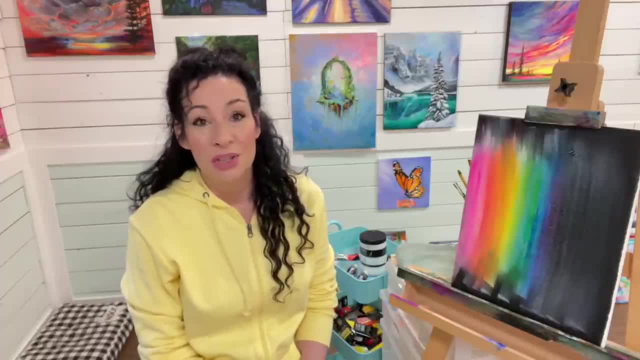 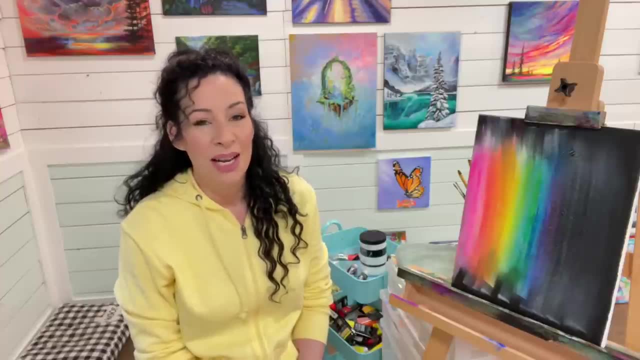 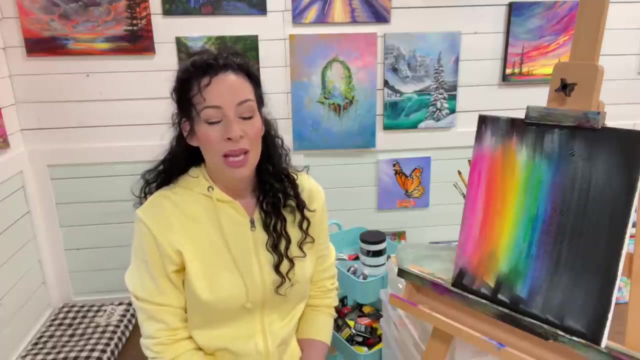 we are as an artist, yet not knowing the next brush stroke to take, the next thing to paint- uh, it can be really frustrating. a lot of paintings get thrown out in the trash or painted over. it happens. so what I've learned over the years and my tips and tricks for overcoming that and getting through is: 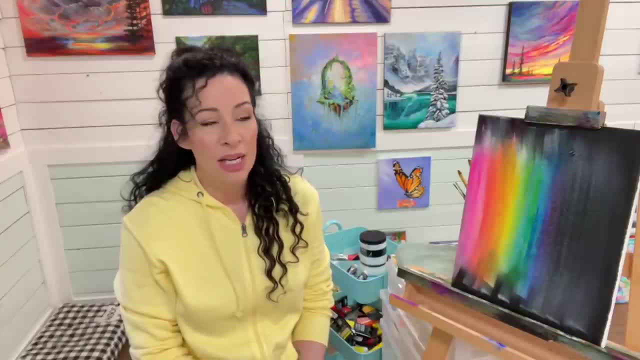 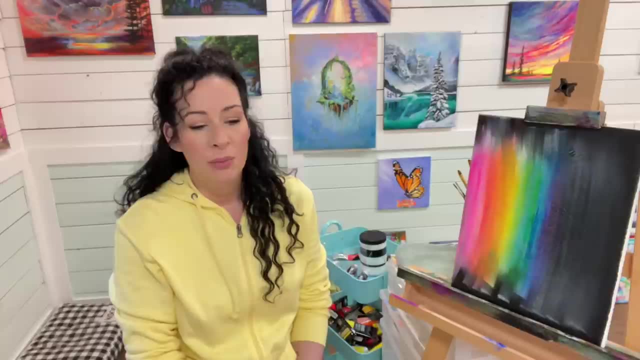 something's going on in your life and you're upset, you're or you're angry. it's subconsciously, without you're realizing it or doing it on purpose. it's going to come out in your painting, um, so I I'm just telling you guys what works for me and what could help you. I'm giving you my tips, right? so? 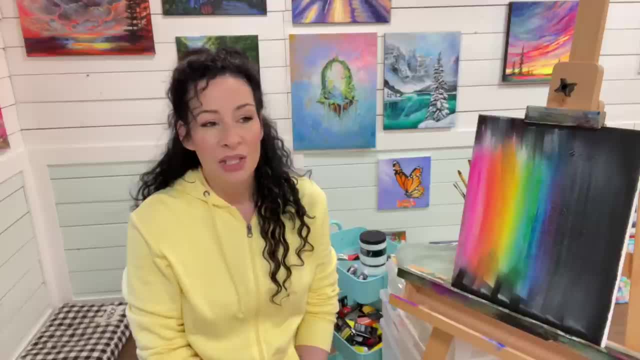 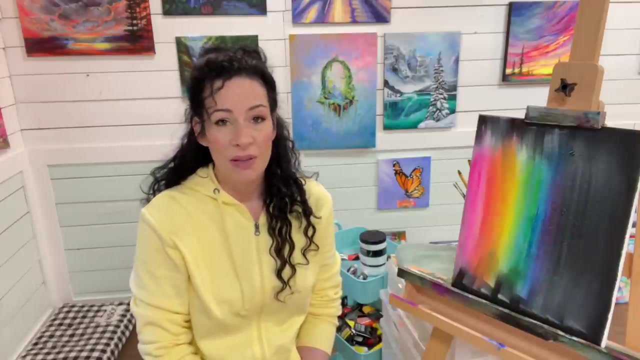 it's different for everybody, but I like journaling. I like to just get out everything that I'm feeling, everything that's going on into my journal, and then I feel like it's, it's out there and it's not going to come out onto my canvas. that being said, art is therapy, so you can get everything out onto. 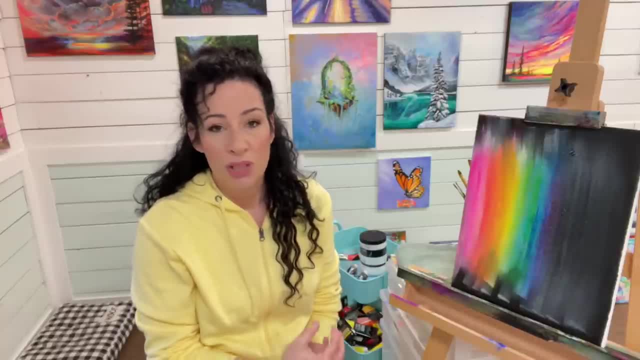 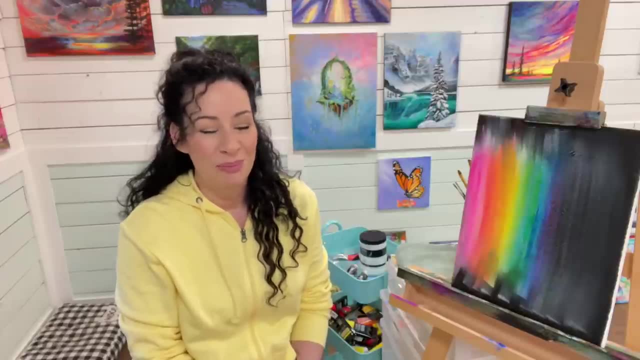 your art and color, but if you're trying to create a landscape or a specific image, then it it's. those are two different things. it's like apples and oranges, so there is art therapy for sure. um, a few other things that I like to do. I like to make sure that I'm getting outside for brisk walks. 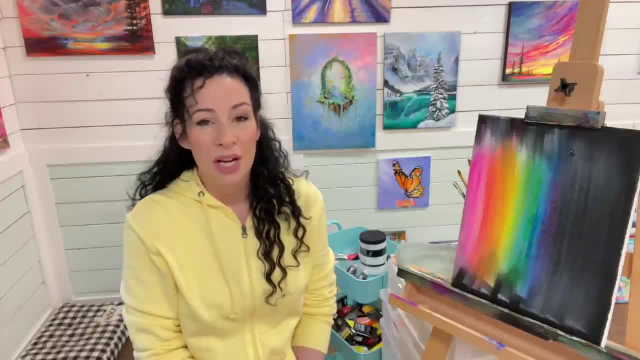 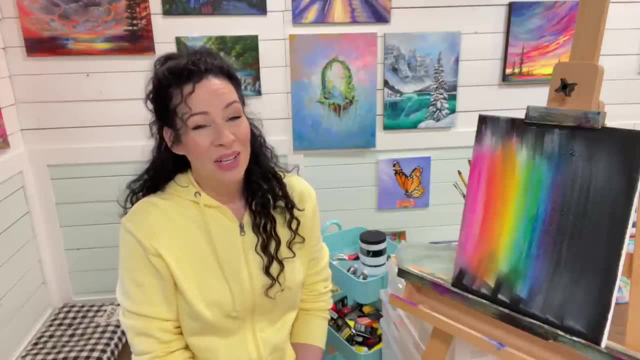 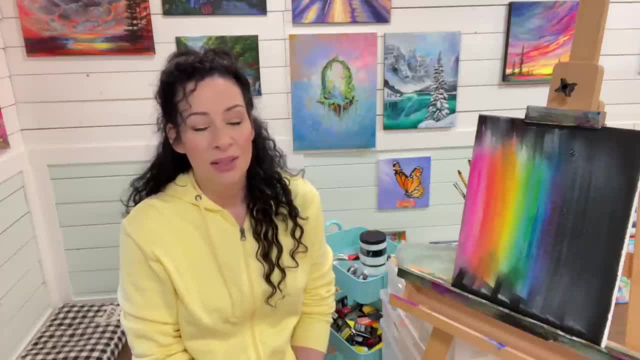 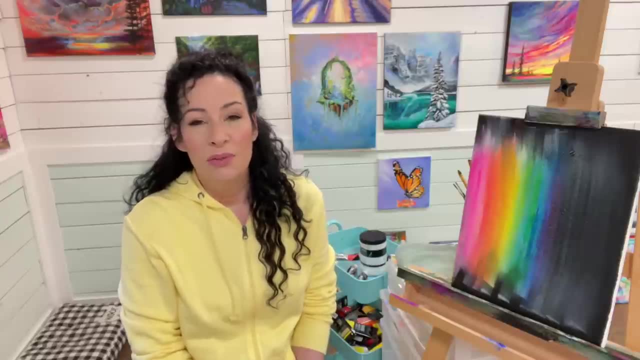 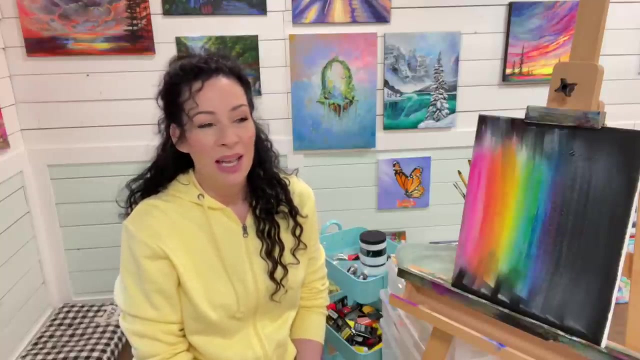 by the ocean, so that's really made me a much happier and more content artist as well. um, and I also like to listen to relaxing music, so whatever music that uh makes you feel good, you know anything that gets your serotonin up, um, a cup of coffee, a nice cup of tea, music, anything. 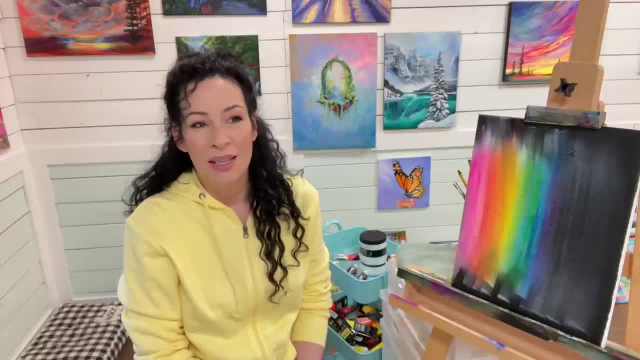 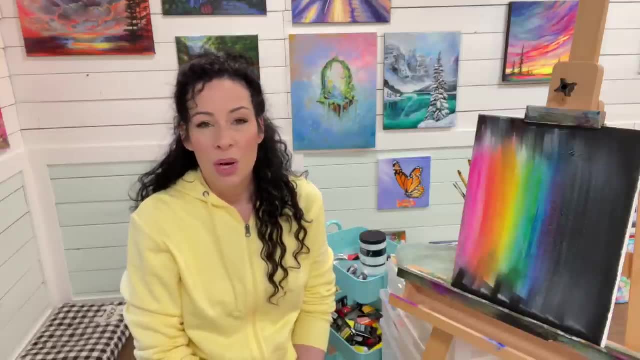 you know, uh, just getting your your mind in that happy, content, worry-free state of mind, um, and sometimes you know, we don't even know what colors we want to use, we don't what we want to paint, and that can be the biggest part of frustration when you're beginning a. 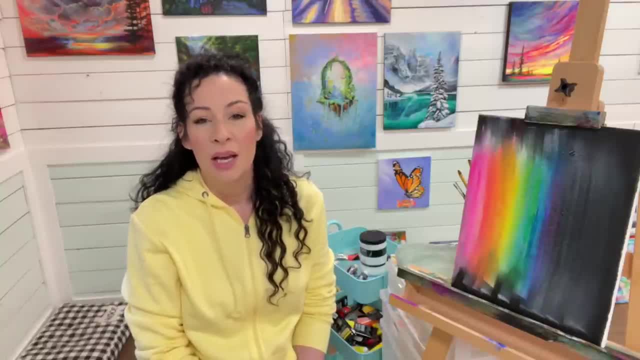 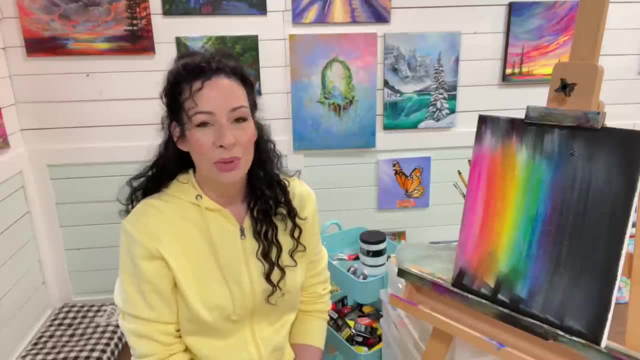 painting is i don't know where to start. you know, you kind of have that, uh, instead of a writer's block that writers get when they're working on a story, we get uh, painters block, don't we? we don't know what we want to paint. so i've- i've had that so much over time, but what i always am drawn to, 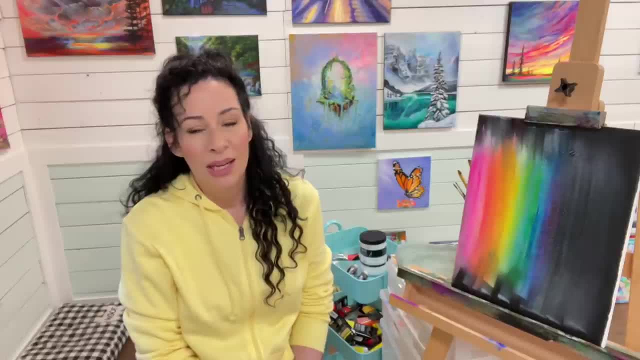 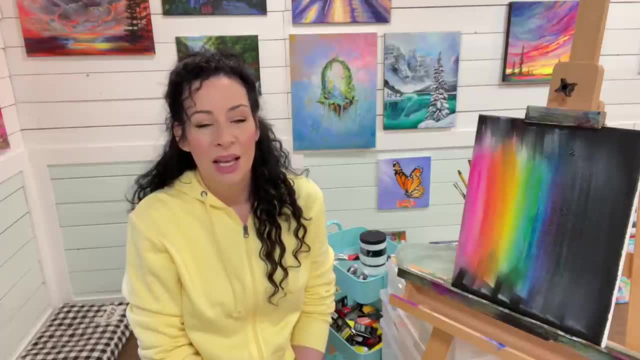 and i always end up doing is, if i don't know what i want to paint, i just go through my my paint colors and i i just pick up colors that are fun and that i like to use and i like to see and um are visually stimulating to me. so i like to go for those bright colors. i love my neon colors. 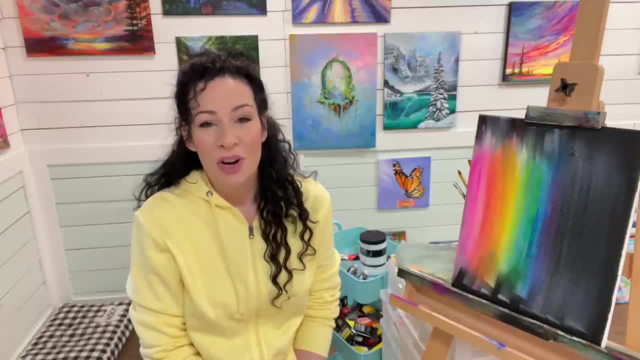 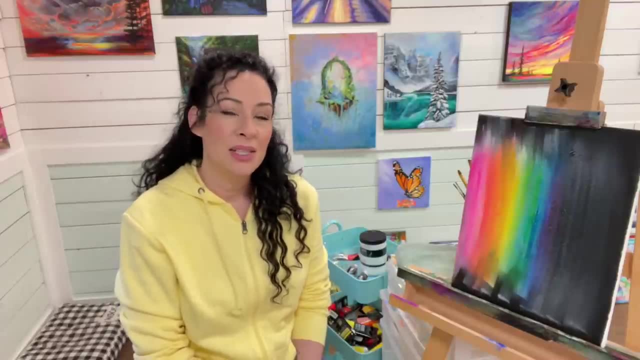 those have brought me a lot of joy and i will just start in an abstract sort of way, kind of just like what that state of mind, if you can remember what it's like to be a child, and i touched um on this a little bit in my last intuitive fantasy painting i did with all the cherry. 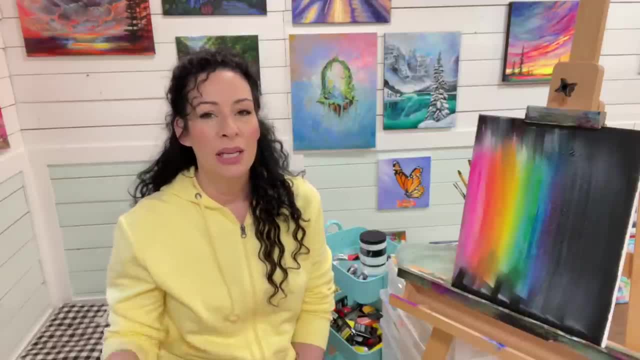 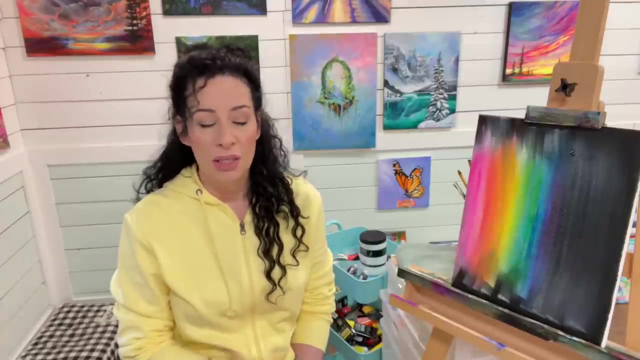 blossoms. i'll leave a link below for that, where i really take you step by step through my what, going through my mind and my process of painting intuitively, so you can kind of understand what i'm feeling, what i'm what i'm thinking throughout my painting process a little bit more. i'll just touch on it a little bit here. uh, i loved color. 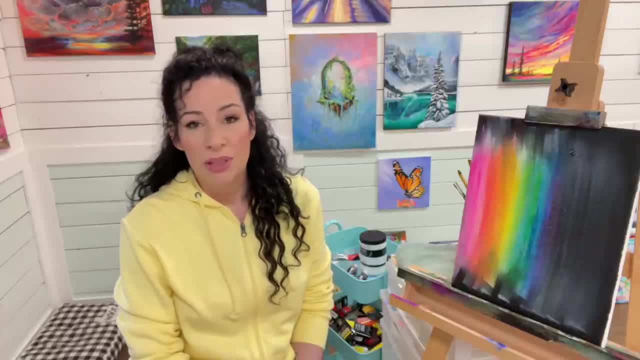 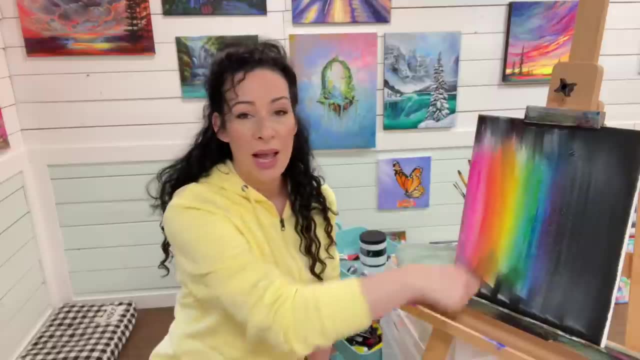 when i was a kid. my mom still has pictures of when i was like three years old and i was doing stuff actually like this. i would take every color of crayon in the box, every single one. i had to use all of them. i couldn't leave any of them out. 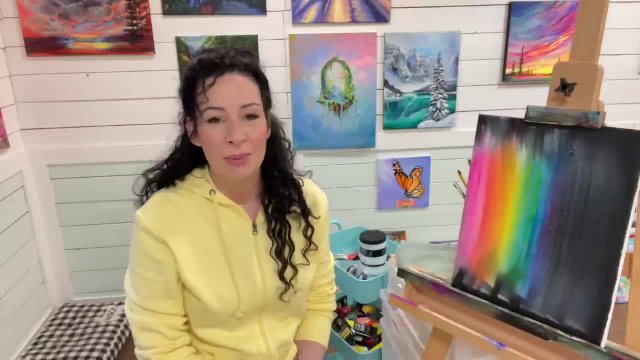 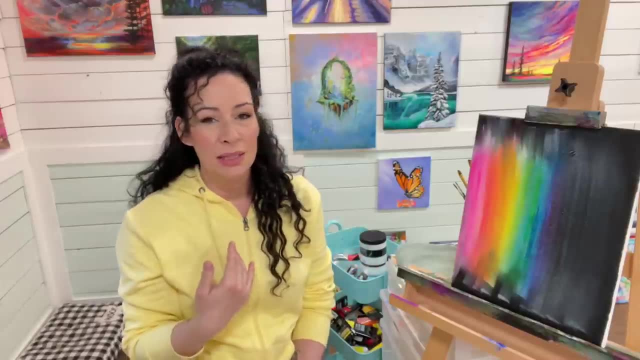 i wanted to see all the colors, so, um, but oftentimes when we start in an abstract way like that and just create patterns and you're calming your mind and your body and your spirit just by doing that, that can get you in that state of mind and it. 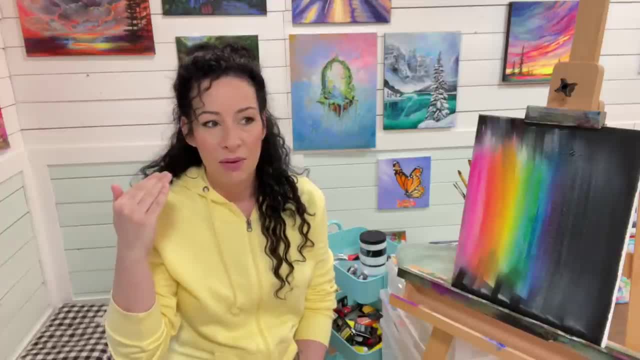 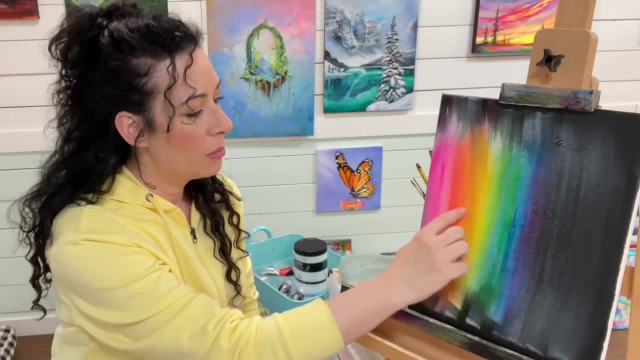 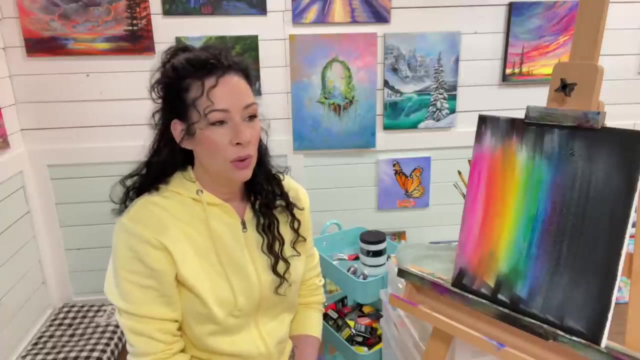 starts, it starts to make you feel more creative and, um, things start to happen. you end up starting to see i could see maybe a little house right there, or maybe there's a waterfall or a tree and we see a tree. that's those start to use our imagination and that's such a healthy thing. So it's actually a good thing if 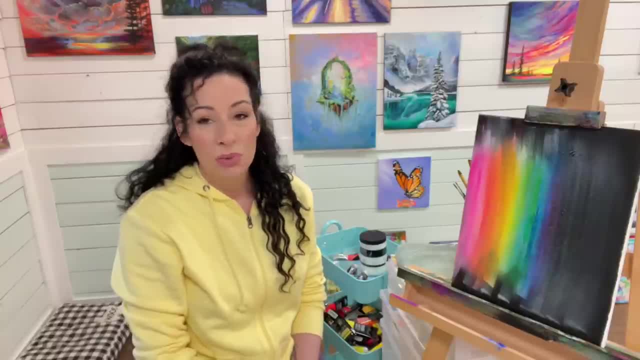 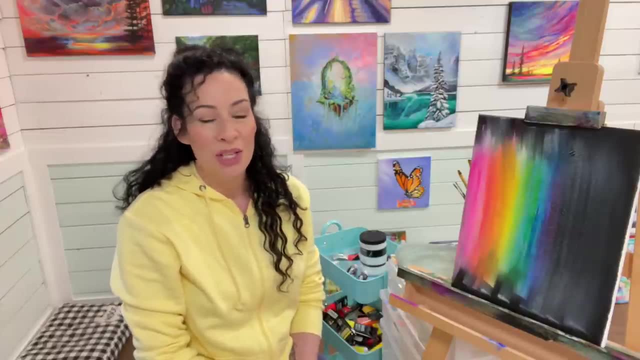 you don't have a reference photo and you don't know what to paint. It's really really good for your mind. It's a nice little exercise to keep your brain healthy and keep those creative juices flowing and your imagination working. So, the blank canvas, not knowing what to do, pick a few colors. 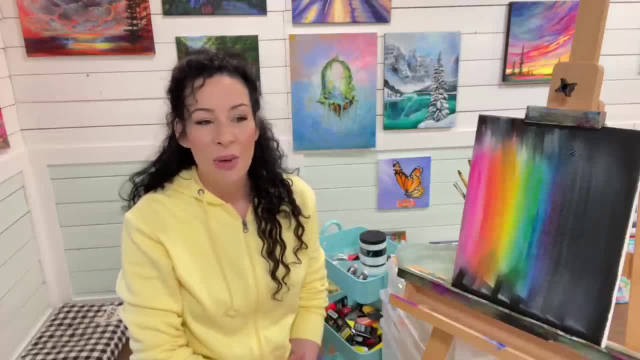 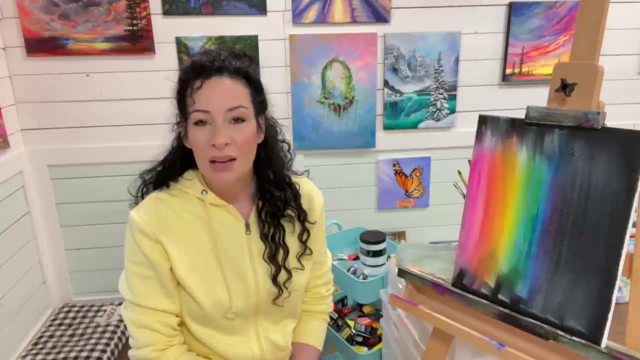 just have fun like you were a kid and you had no expectation. You know, we had no fears when we were kids. We didn't worry about what anybody was thinking. We were just in that state of mind of having fun, and so that's what you want to get back into and that's the best, I think, out of all of. 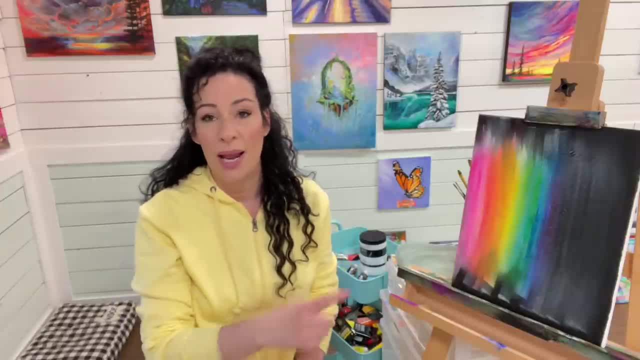 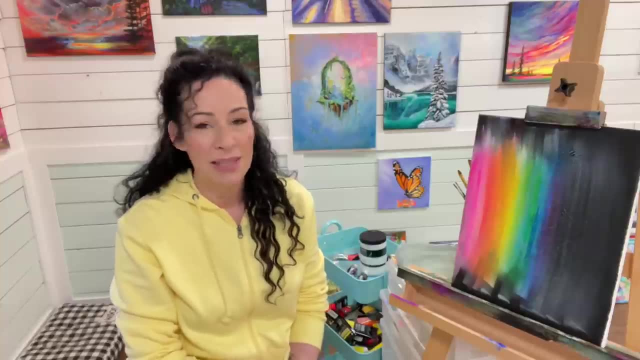 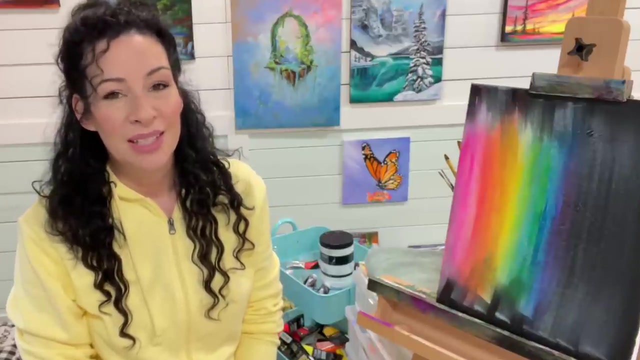 these tips. I think that should be number one before anything else, because it doesn't matter how many tools you have, what you have- the best canvas, the best brushes, the best paint- you can have all that stuff, all the tools, but if your mind's not in a good place and you're